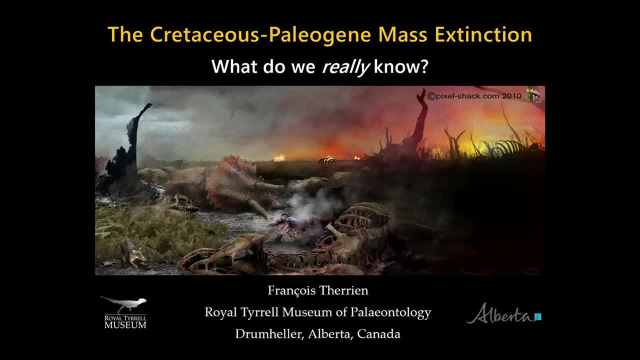 Can you hear me? Yes, Excellent. So the Cretaceous-paleogene mass extinction is probably one of the most talked about topics in paleontology these days, And that's understandable, because that event marked the extinction of the coolest animals that have ever lived- the dinosaurs. 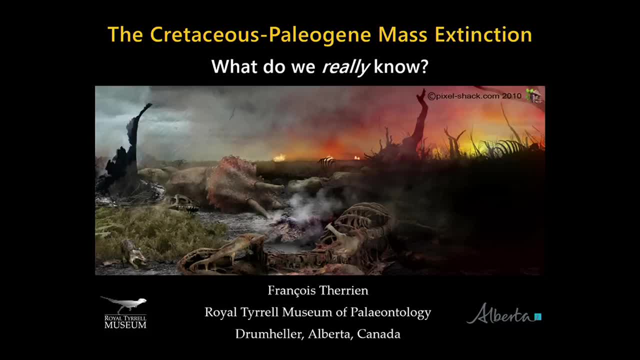 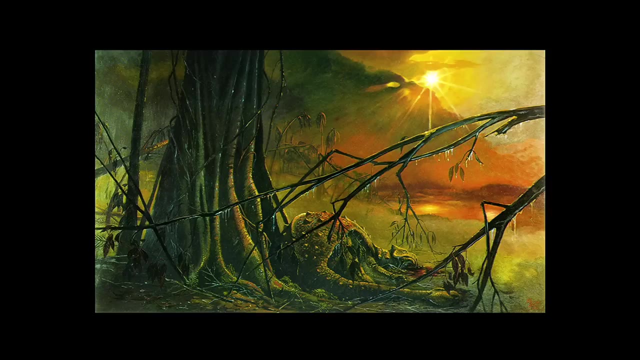 Of course I'm a little biased, but you'll forgive me. So over the years, many theories have been suggested to explain the extinction of the dinosaurs. Well, we have that problem. There we go. So some theories invoke long-term, major environmental and climatic changes. 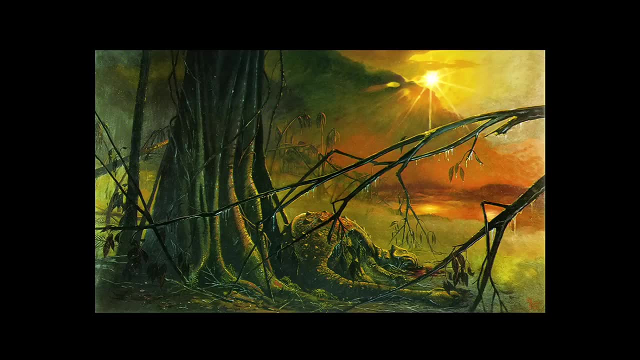 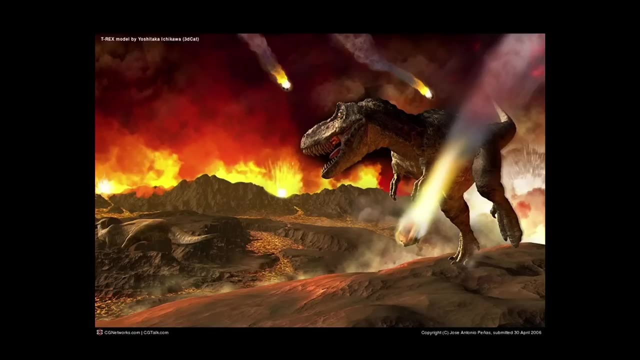 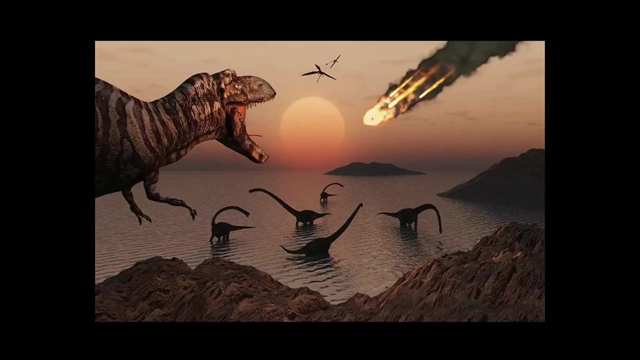 to which dinosaurs could not adapt, that led to their extinction. Other theories invoke major volcanic eruptions that happened at the end of the Cretaceous, that polluted the atmosphere, affected climate and killed off the dinosaurs. And then there's a theory, probably the most common, the most popular one. 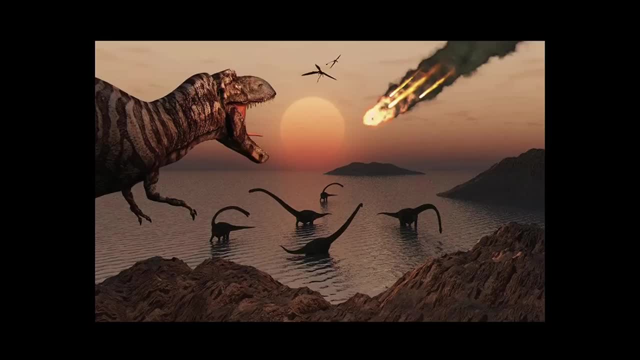 is that of a meteorite impact that happened at the end of the Cretaceous that created major environmental disturbances leading to the extinction of dinosaurs. There's also a few more theories that are a little bit more exotic. For example, there's a theory that was claiming: 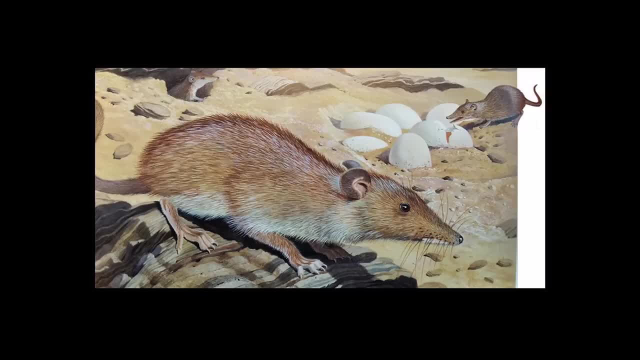 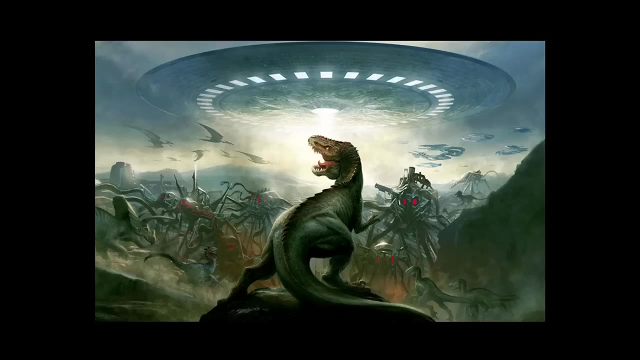 that those furry, pesky little mammals actually got hungry, started eating some of the dinosaur eggs, and dinosaurs could not bear offsprings, and that led to the extinction of dinosaurs. There's also theories that invoke some extraterrestrial beings kidnapping dinosaurs. 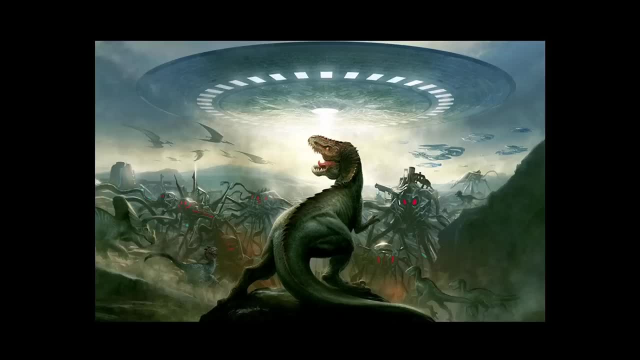 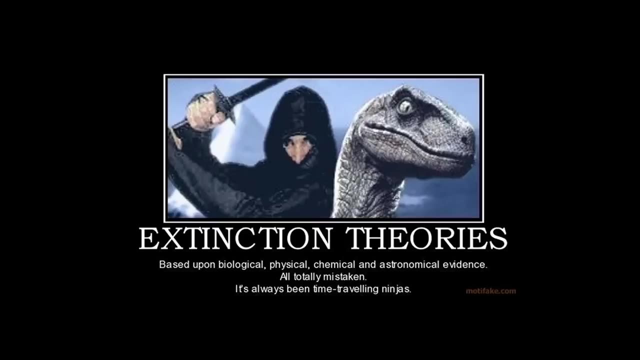 bringing them to their home planets for zoos. And then a theory I came across on the Internet that I find really, really interesting is that mass extinctions would actually be related to time-traveling ninjas, which is actually really cool, I think. 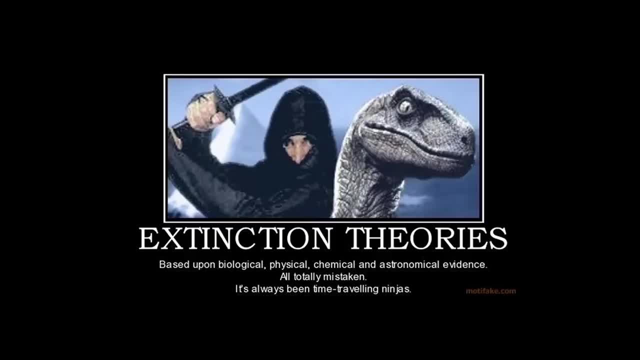 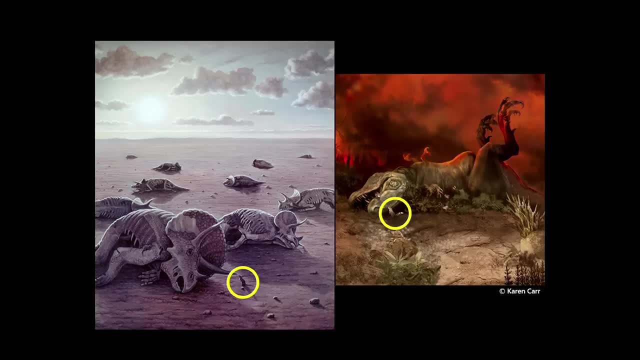 So, regardless of which theory you prefer, they all have one goal in common: They all aim at trying to explain why dinosaurs went extinct when the small little mammals survived. So in my talk today, I'll give you an overview of what we know about the Cretaceous-Perigene mass extinction. 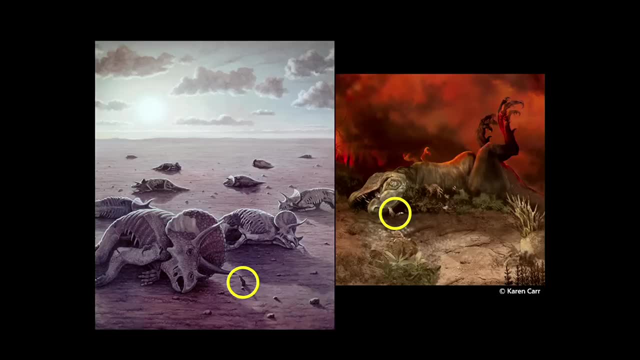 present some of the latest developments- some were published just last year- on what we know about the extinction event and finally conclude with a scenario of the possible cause or causes for the extinction of dinosaurs. But let's start with a little bit of background information. 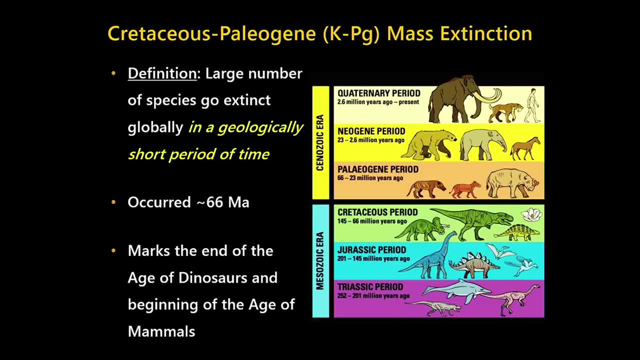 First let's define what is a mass extinction. So a mass extinction is when a large number of species goes extinct globally. so this means it occurs all around the world, but also in a geologically short period of time, And that's a key word. 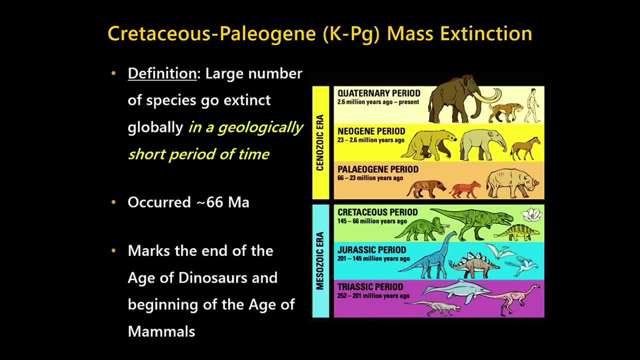 geologically short period of time. This means that the extinction does not need to happen overnight, in a year or even over a century. It just means that it happens at a time scale that makes it difficult for us to resolve using the stratigraphic record. 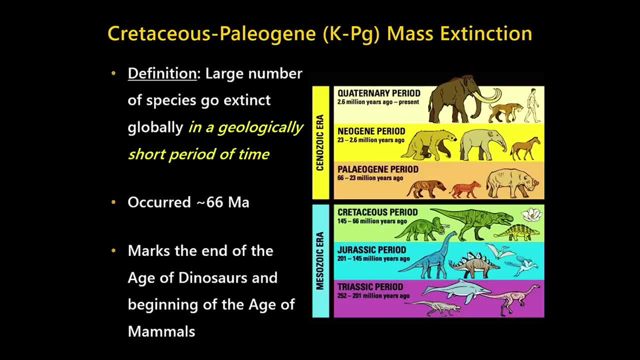 So if we go back 66 million years ago, at the end of the Cretaceous, resolving an event to within 100,000 years is pushing the limit of what we can do with our current fossil record. So when we're talking about geologically short periods of time, 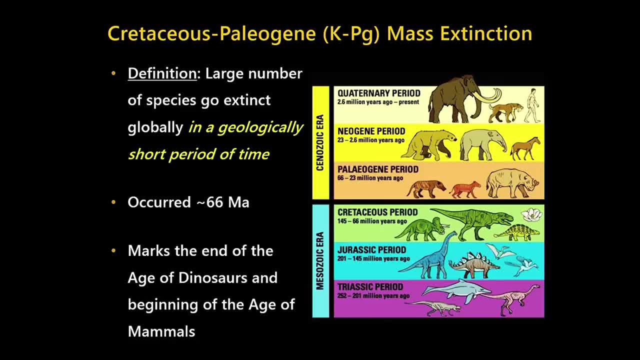 it's all a relative meaning. So the Cretaceous-Paleogene mass extinction, or KPG for short, or you've probably also heard it referred to as the K-T boundary extinction. it occurred roughly 66 million years ago. It occurred at the boundary 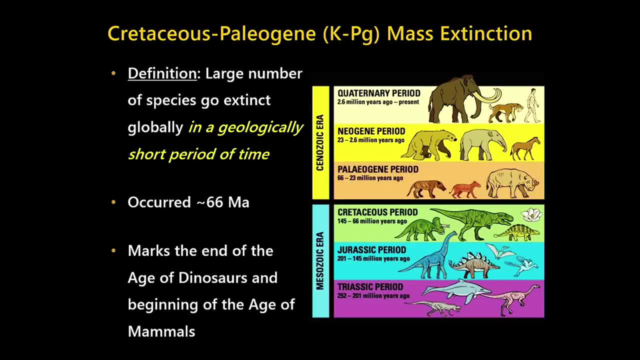 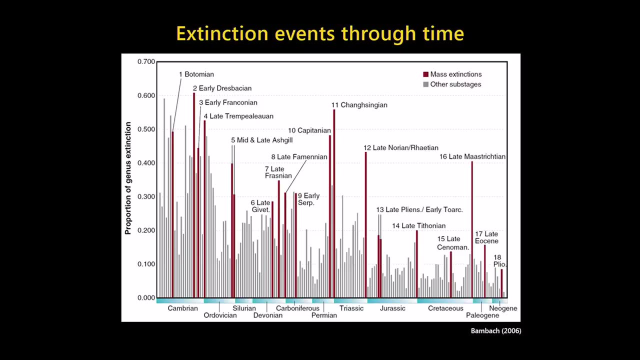 between the Cretaceous and Paleogene periods, so you'll often hear me refer to it as the KPG boundary- And that extinction marks the end of the age of the dinosaurs and the beginning of the age of mammals. So the KPG mass extinction might be. 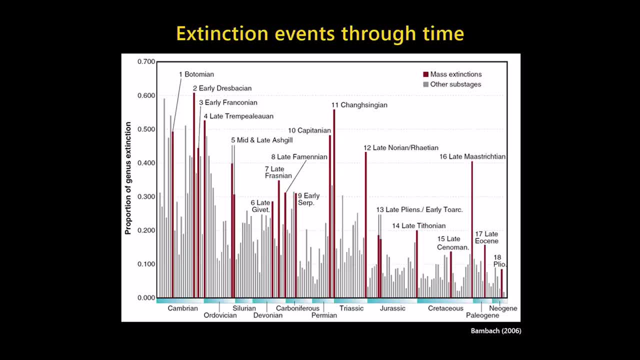 the most famous of mass extinctions, but it's far from being the only one. If we look at a graph of extinction over time over the last 600 million years, we can see one thing right away is that extinction happens all the time. 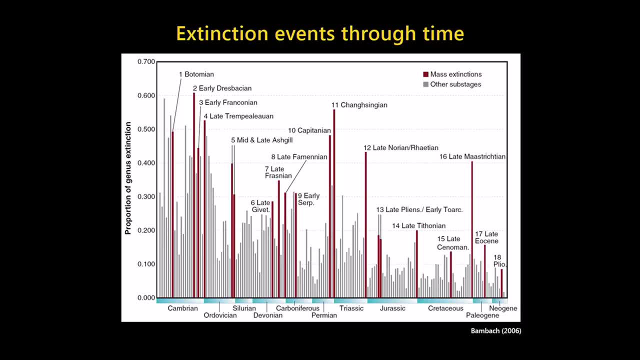 Every time we have species that go extinct or replaced by other ones, but it happens regionally, not globally, or it happens over a longer period of time. So those are background extinctions and that's a common course for life. But there's at least 18 different events. 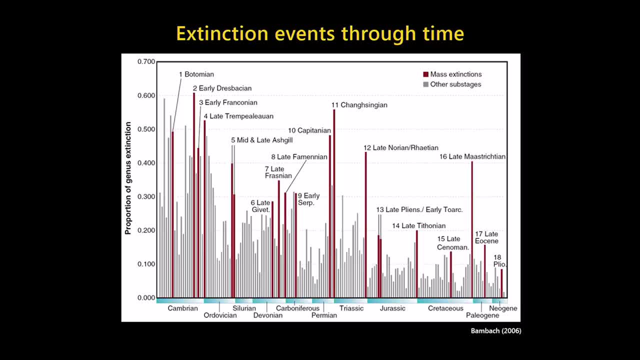 or instances over the last 600 million years where species went extinct rapidly and globally. So that means those qualify as mass extinction events And there's a study that came out just last year suggesting that we're actually entering the beginning of a 19th mass extinction right now. 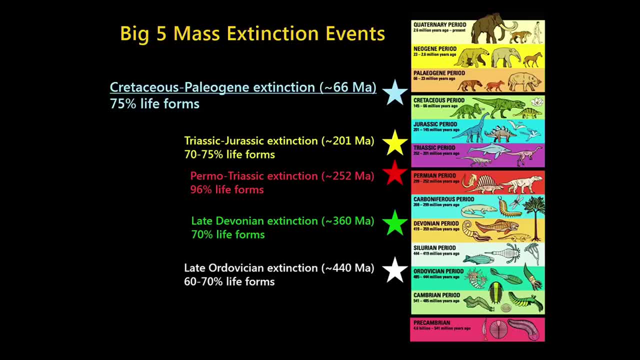 So out of all those 18 mass extinctions, we usually talk about the big five mass extinctions that have been cherry-picked based on the percentage of life forms that have gone extinct. So we can see that the KPG mass extinction is not the biggest one. 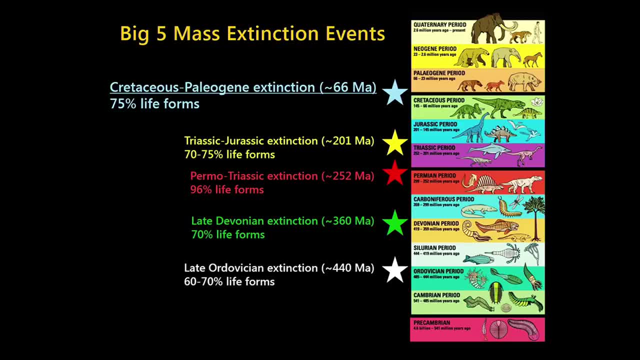 The Permo-Triassic is responsible for 96% extinction on Earth, But the KPG mass extinction is arguably the one that had the most direct impact on the nature of the world in which we live today. So without the KPG extinction, 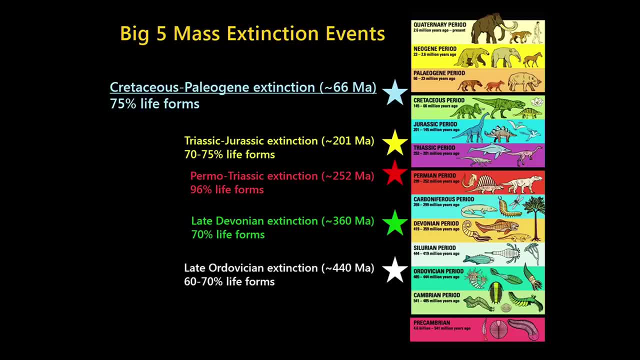 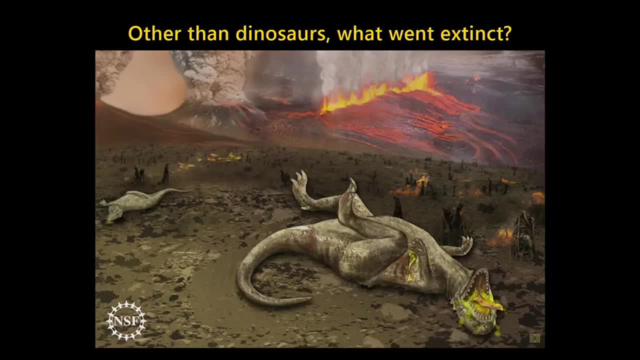 a world dominated by mammals in which our species could have evolved would probably have never occurred. Dinosaurs are obviously the poster children for the KPG mass extinction, but they're far from being the only organisms that have gone extinct at that time. There's lots of plants and animals. 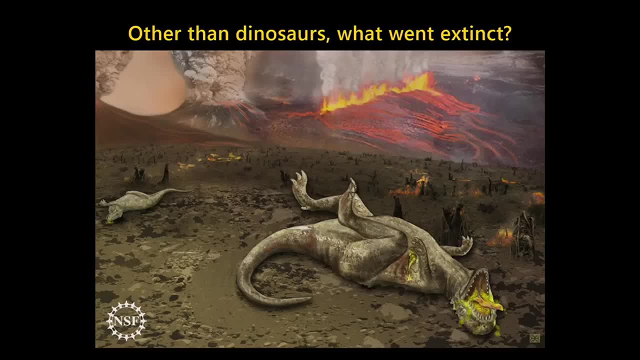 that have gone extinct both on land and in the ocean, And we'll have a quick look also right now at what other animals went extinct alongside the dinosaurs. So first, if we start in the oceans, we can see that the KPG extinction. 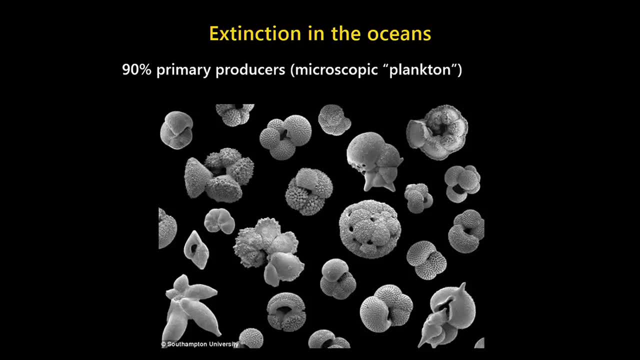 claimed 90% of the primary producers. So this means primarily the plankton that lives in the oceans. So the plankton is the base of the food web on Earth. They're responsible for the majority of the oxygen we breathe. So by wiping out 90% of the primary producers, 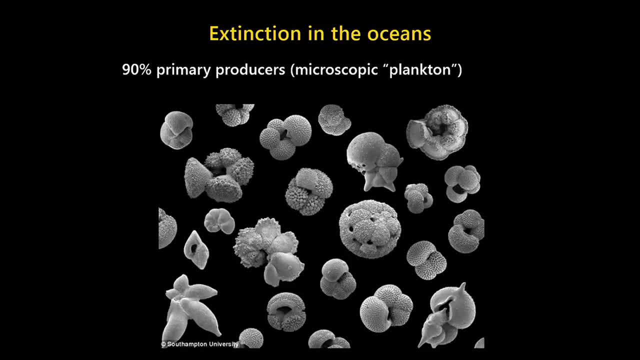 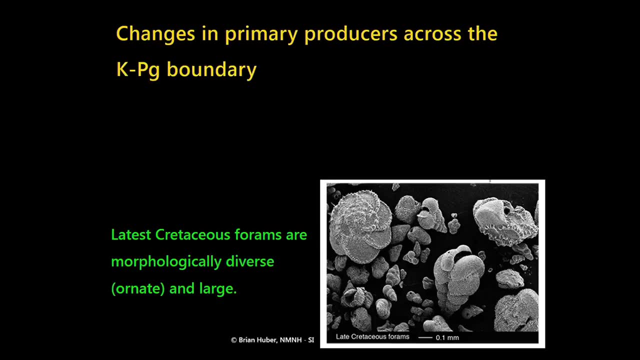 the mass extinction just destroyed the base of the food web on Earth. But not only did the mass extinction claim a lot of plankton, it also affected the survivors for many millions of years afterwards. So here's a little slide showing what foraminifera small planktons 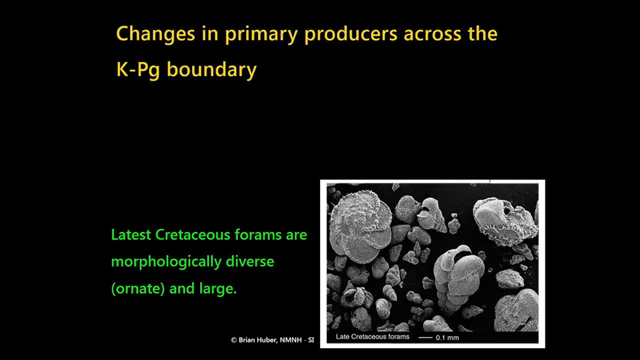 of the late Cretaceous, what they looked like just before the Cretaceous-Pelogene boundary. We can see they're highly diverse in shape and in size. Some of them got relatively big. It's all relative because you can see the scale bar is only 0.1 millimeters. 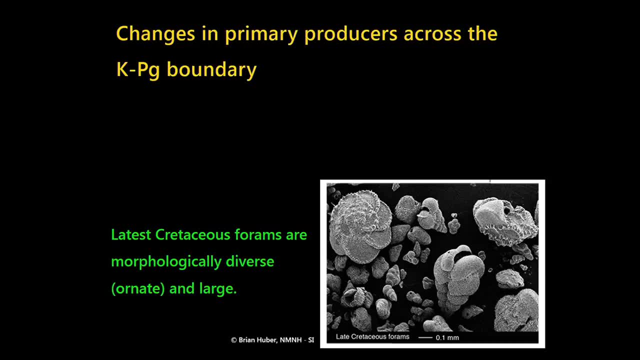 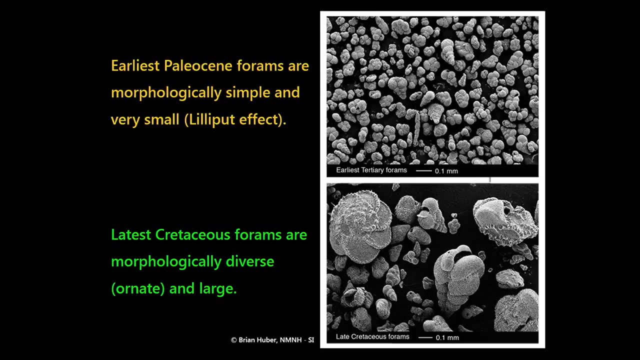 But you can see, some of them are bigger than others and there's lots of ornamentation, so they're highly diverse and specialized. But right after the boundary we can see that the forearms have changed dramatically. They're definitely much, much smaller. 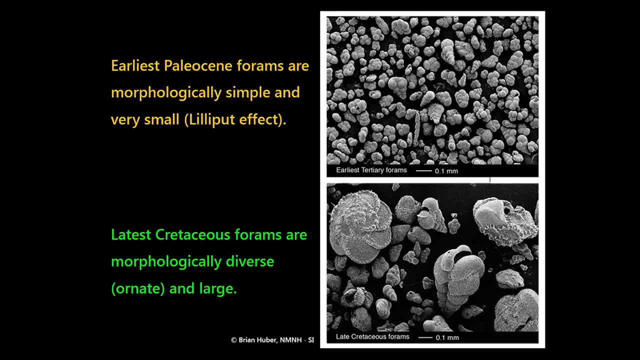 and they're a lot less complex, less ornamented. So that's telling us that the conditions in the oceans were really stressed, really bad for growth of plankton, and that lasted for at least 4 million years after the extinction event. 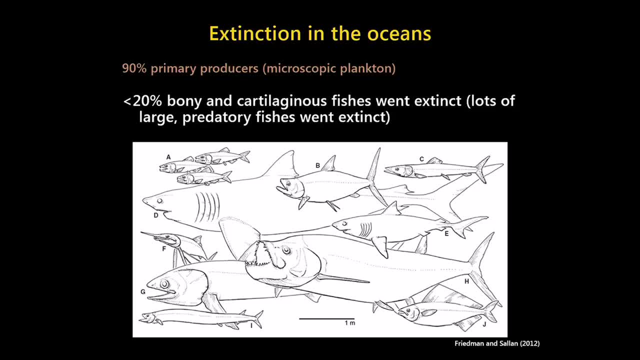 If we look at fish, surprisingly most fish fared pretty well across the boundary. There's only a less than 20% extinction. but the species that have gone extinct are usually the large, fast-swimming predatory fishes. So the large Xiphactinids have gone extinct. 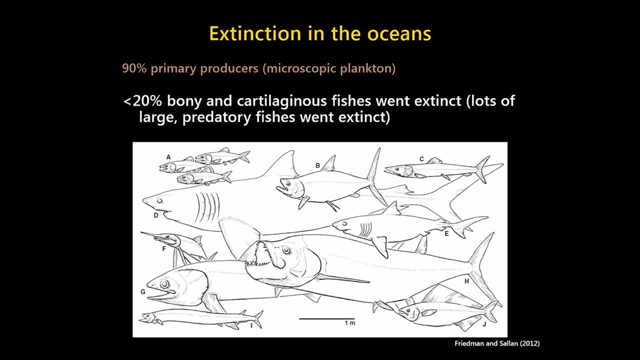 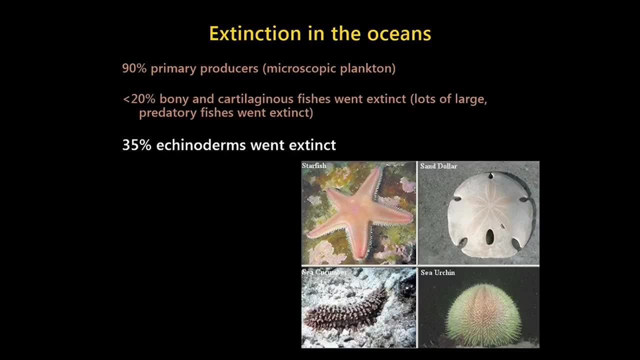 Lots of large sharks also went extinct, But otherwise the smaller fish went through the boundary unscathed. If we look at the echinoderms, so starfishes and sea urchins, we see a little bit of extinction in these animals. 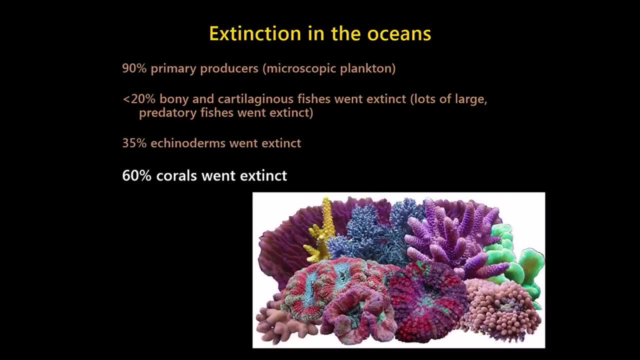 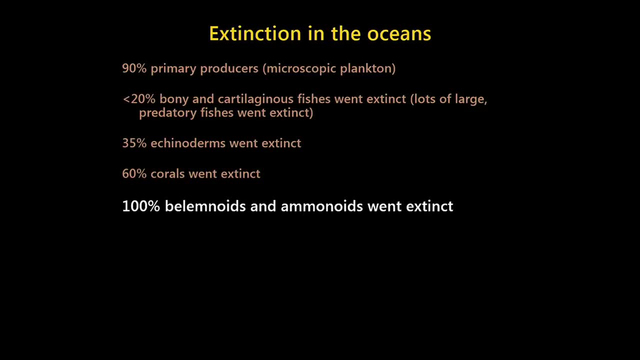 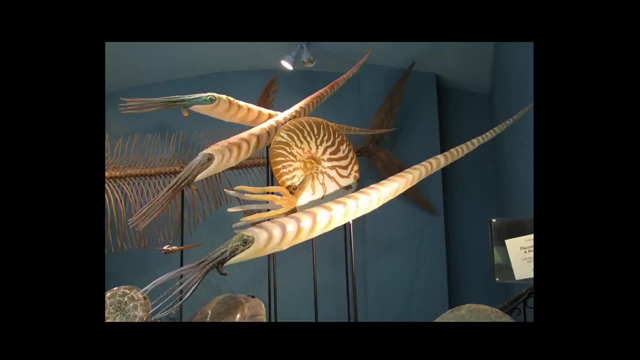 but corals suffered a lot more. Over 60% extinction happened among corals. Then we have animals that were totally wiped out by the extinction. That includes the bilaminoids and the ammonoids. Those are squid-like animals that lived in straight shells or coiled shells. 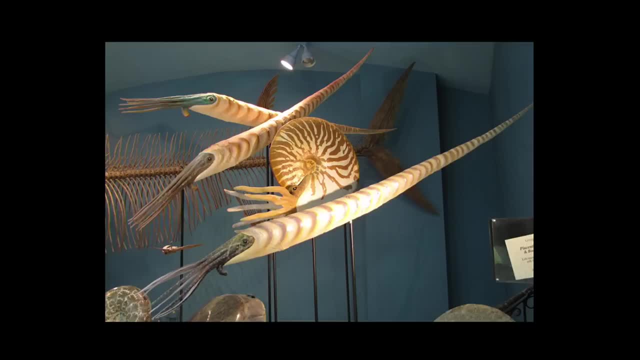 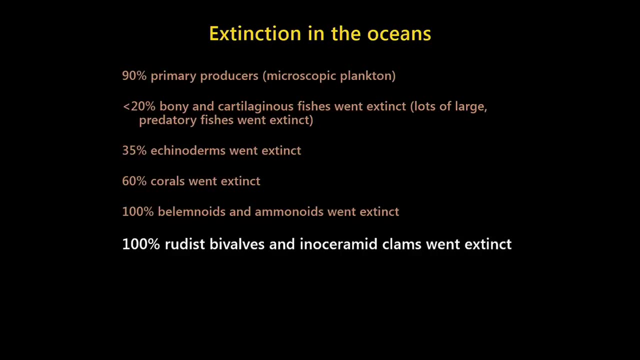 They were really abundant during the Mesozoic. They lived in oceans all around the world, But at the end of the Cretaceous they all went extinct. We also see the extinction of rudis bivalves and inoceramid clams. 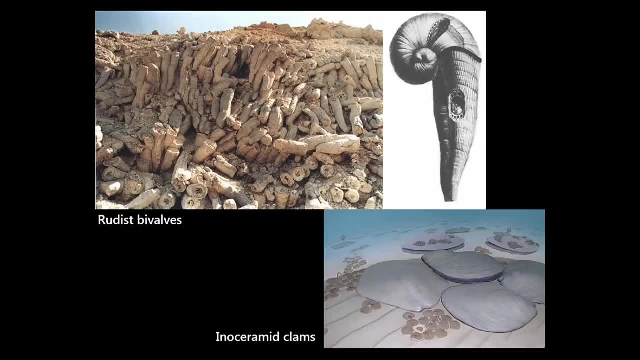 Those are mollusks. You can see. rudis bivalves are weird columnar clams that actually formed reefs. And those rudis have actually an economical significance, because most of the oil reserves in the Middle East are actually trapped inside those rudis reefs. 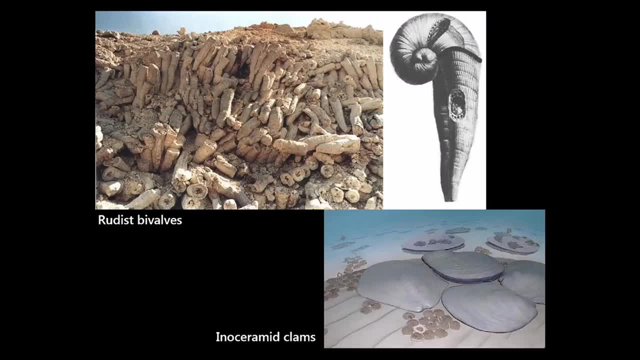 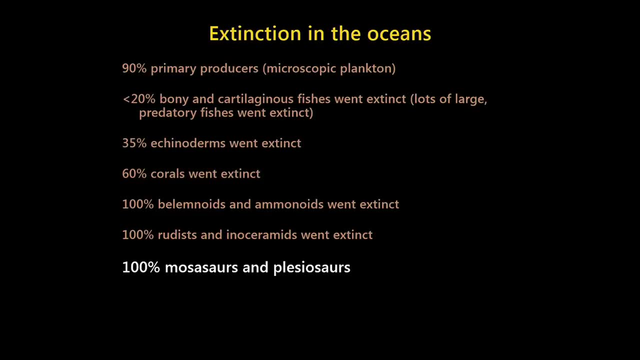 And then we have inoceramid clams, which are large shells that could be up to 2 meters across. So those also went extinct. And then, finally, we have the mosasaurs and the plesiosaurs that have gone extinct. 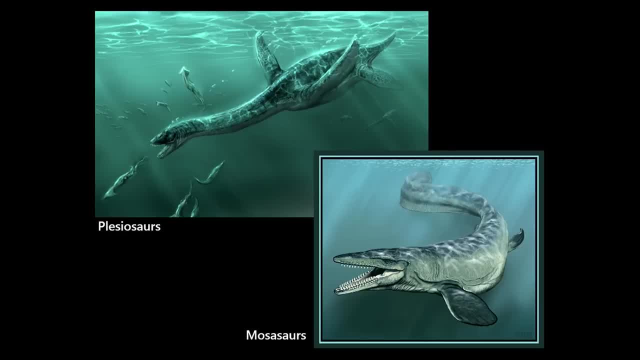 often erroneously called marine dinosaurs, These animals are actually not even closely related to dinosaurs. Mosasaurs are marine lizards closely related to snakes and Komodo dragons, whereas plesiosaurs are long-necked marine reptiles distantly related to the ancestors of snakes and lizards. 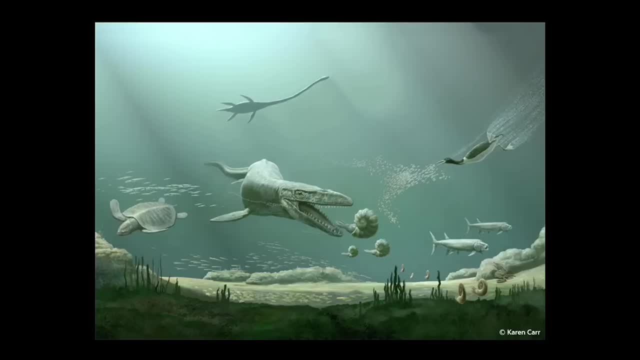 So if you were to go snorkeling or scuba driving in the ocean just before the K-Pg boundary, that's the kind of animals you'd be swimming alongside, So it would have been a pretty terrifying but interesting activity. But then if you went back and went swimming, 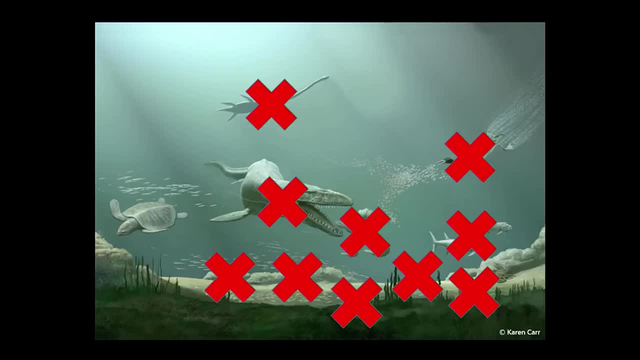 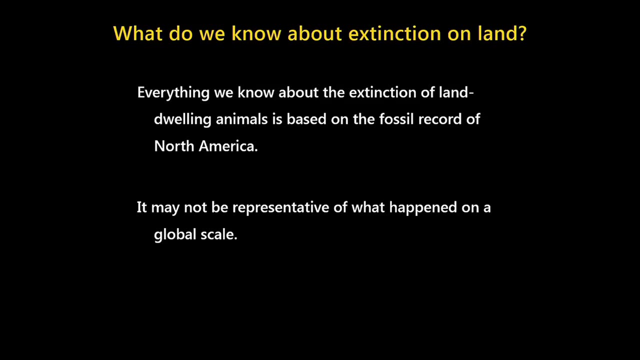 after the extinction, you'd see that most of those animals would be gone and the oceans would look relatively empty. in comparison, What do we know about the extinction of animals on land? Well, we know actually very little. The only record we have for the extinction of land-dwelling animals 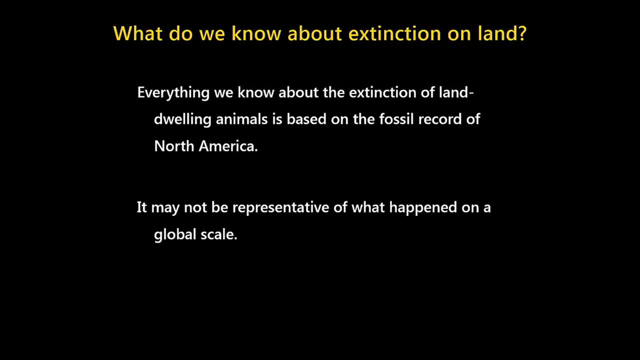 is based on the fossil record of North America, primarily of Montana and the Dakotas. Nowhere else on Earth do we have any record for the K-Pg transition, or the fossils have been poorly documented to date. So I'll discuss here a little bit of a pattern. 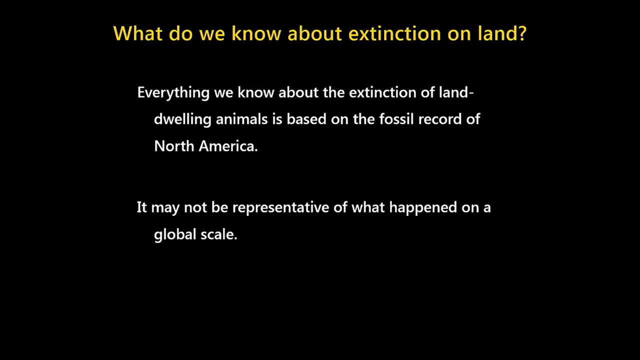 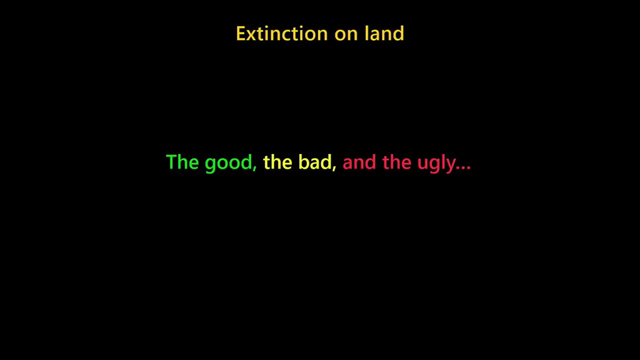 of extinction we see here in North America, but keep in mind that this may not actually be a representative of what went on around the world. So when we look at the extinction of terrestrial animals, we see that some animals went through the boundary event without any problems. 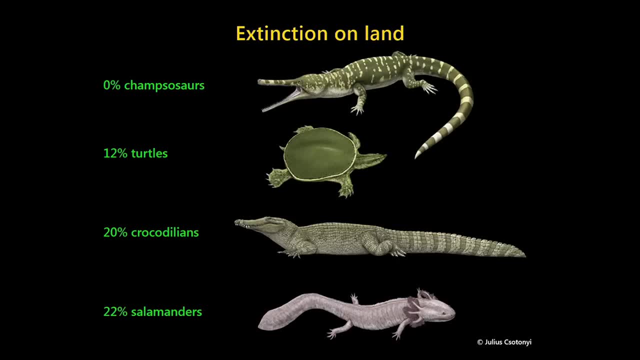 whereas some others suffered tremendously. So if we look at animals that were relatively unscathed by the Cretaceous-Paleogene boundary, we can see we have champsosaurs, Those are, crocodile-like reptiles, Turtles, crocodilians and salamanders. 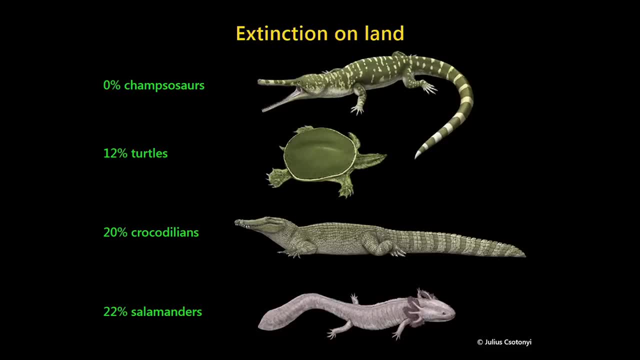 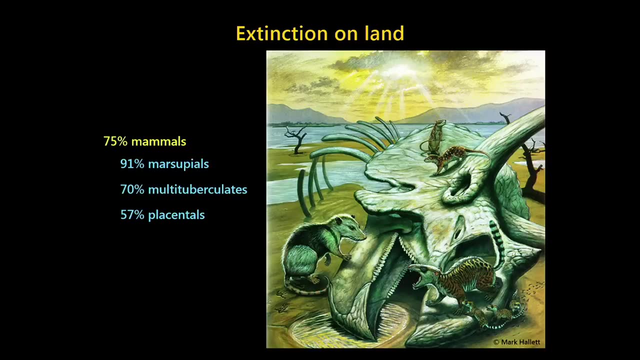 All these animals have very low extinction levels, so they survived the boundary without too much problem. Then, if we look at animals that were heavily affected, we find the mammals. That might come as a surprise to some of you, because mammals are usually presented as being the big winners. 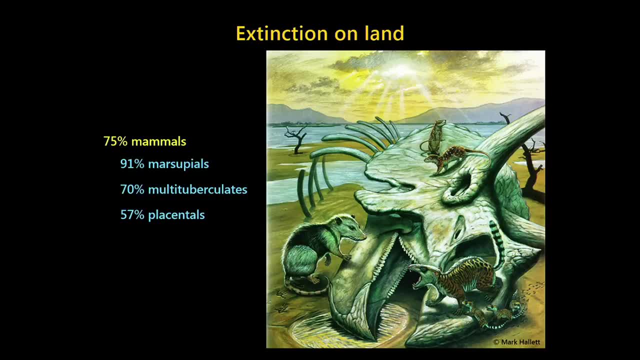 the big survivors of the K-Pg extinction. but we can see actually based on the numbers, mammals suffered tremendously and depending on what type of mammal you were, you were almost entirely wiped out. So it's actually interesting to see that mammals were also victims. 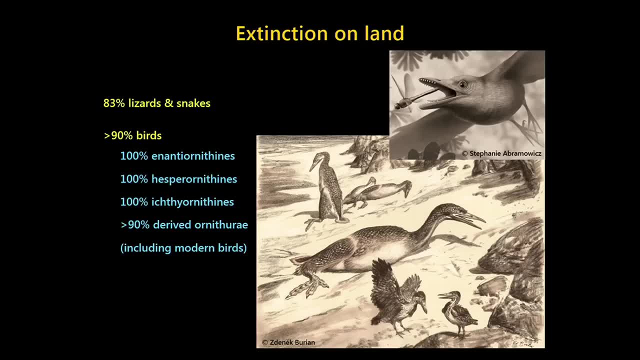 of that mass extinction event. Lizards and snakes also suffered a lot, Lots of extinction- 83%. Birds also suffered tremendously. I put 90%, but that's just an estimate because we have very poor graphs on the fossil record of birds at the end of the Cretaceous. 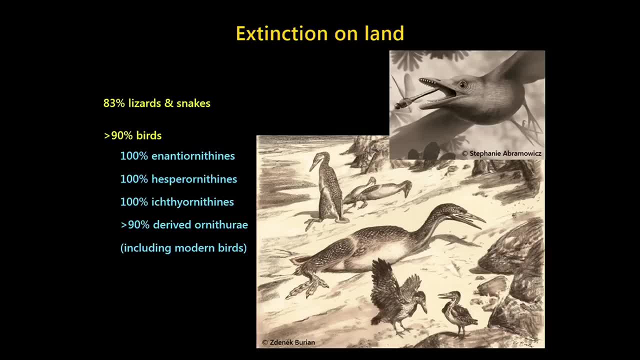 Most of the bones are highly fragmentary so we can only make generalization about the diversity of birds at the end of the Cretaceous. But we can see that some lineages were totally wiped out. Entheornithines- those were the most abundant birds. 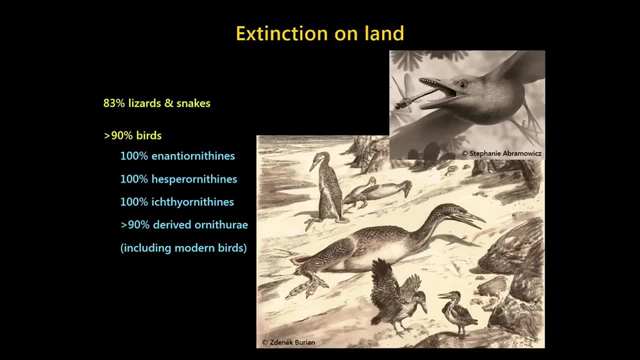 during the Cretaceous. They had teeth and totally went extinct. The loon-like hesperornithines went extinct. Ectheornithines are seagulls with teeth. They went extinct And then among the more derived birds. 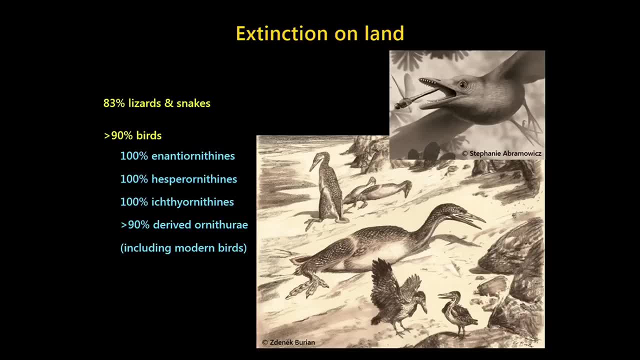 we only have three lineages of modern birds that survived: The lineage leading to ostriches, the lineage leading to ducks and chickens and the lineage leading to all other birds. So we don't know exactly how many species survived, but most birds went extinct at the K-Pg boundary. 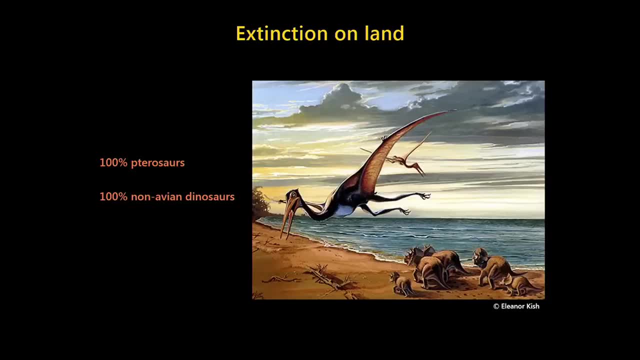 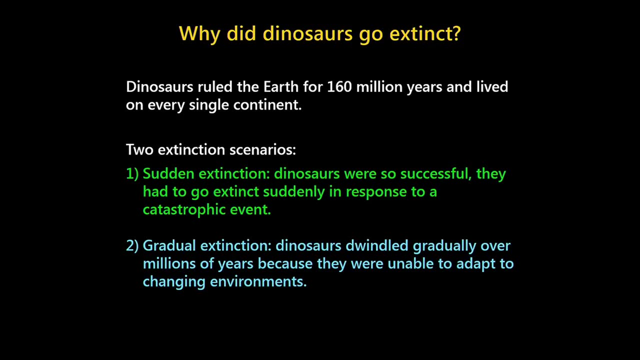 And finally we have animals that were totally wiped out. That includes the flying reptiles, the pterosaurs and all non-bird dinosaurs. So because dinosaurs had been on Earth for over 160 million years, their extinction generated a lot of interest. 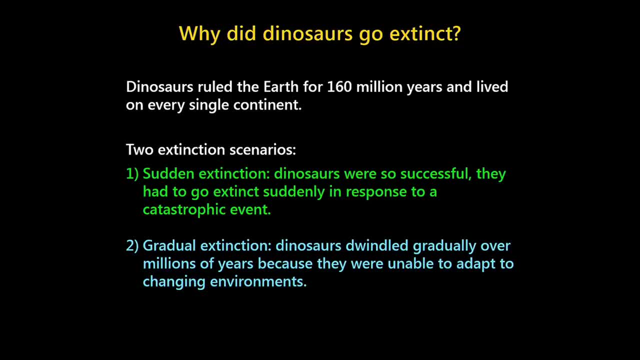 People wanted to know how could these animals go extinct. So there's been a lot of research on the topic and usually theories vary between two extremes. One camp thought that because dinosaurs had been so successful all over the world for so long, the only way they could have been wiped out 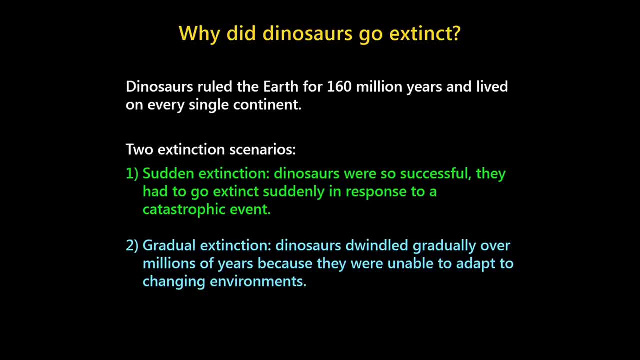 is if a sudden catastrophic event had happened to basically kill them off, Whereas there was the other camp who thought that they could see evidence of a gradual decline over several millions of years in dinosaur diversity, that their numbers were dwindling down as we got closer and closer to the boundary. 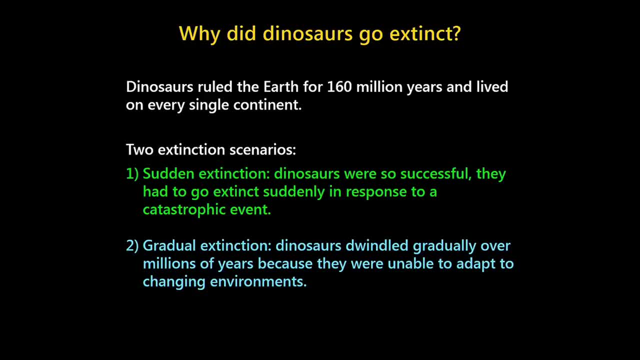 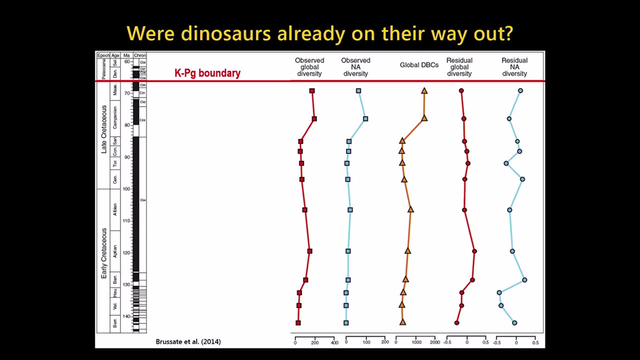 and they went extinct gradually. So that debate has been going on for several decades. But two years ago there was a paper that was published that I think makes a very strong argument for a sudden-extinction dinosaur. So in that study the researchers decided to compile 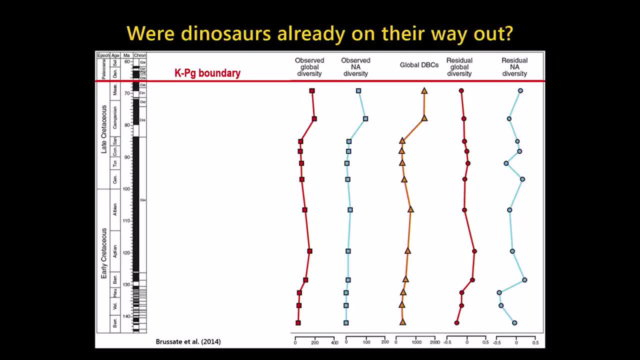 data information about the diversity of dinosaurs both in North America and around the world. So here they plotted features and a few graphs. The two lines we'll just look at are those. It plots the diversity of dinosaurs through the entirety of the Cretaceous. 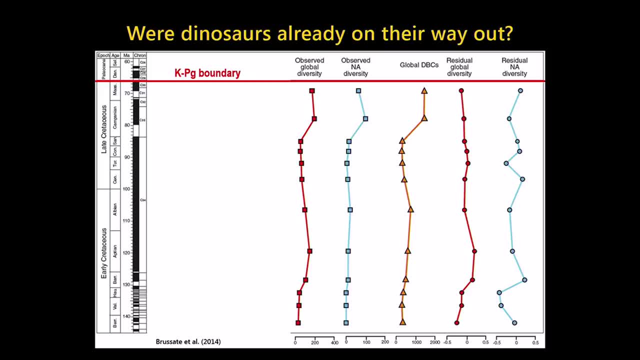 so the last 80 million years of the age of the dinosaurs, And you can see that there's very little fluctuation through time. so it seems to indicate that there is no evidence of a long-term decline in dinosaur diversity over the last 80 million years. 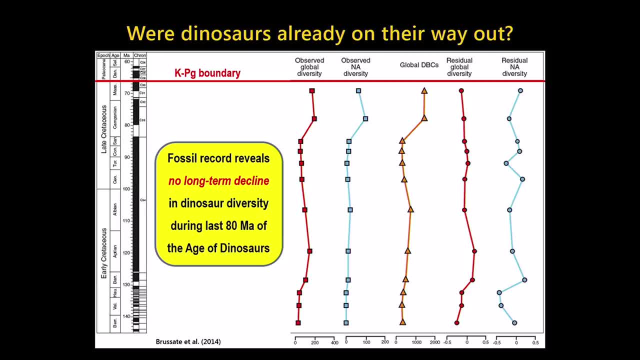 of the end of the Cretaceous. They noted that there was a small decline in North America in the diversity of hadrosaurs in the Cretaceous and Cretopseans, but elsewhere in the world diversity is actually stable or might actually even be going up in some instances. 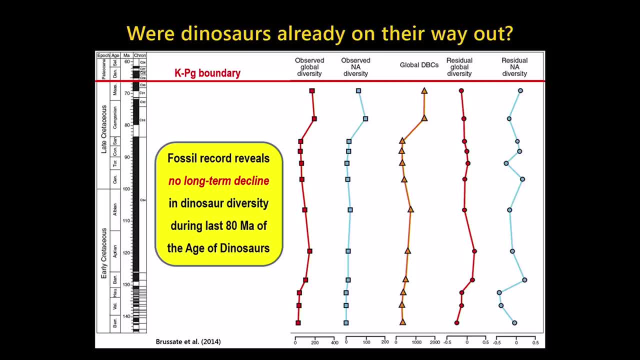 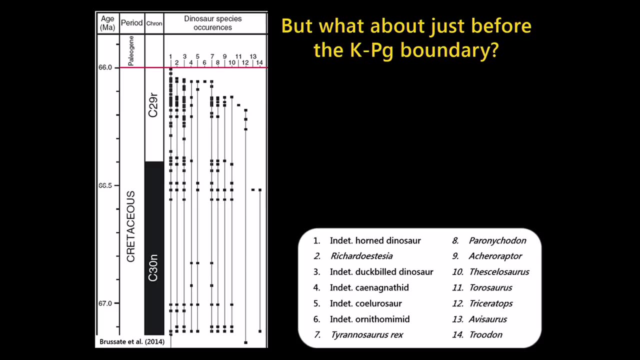 So that's really interesting. It shows that dinosaurs were not gradually dwindling down over several millions of years leading up to the boundary. But what about an extinction? a gradual extinction in the last few million years just before the boundary? So for that they turned to the best fossil record. 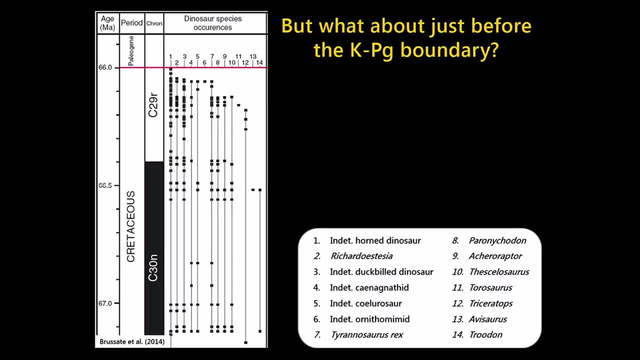 we have for dinosaur diversity, the Williston Basin in North Dakota. There, every dinosaur fossil that's been collected has been. actually the distance from the fossil to the K-Pg boundary has been measured in order to get an estimate of how long before the extinction event these animals lived. 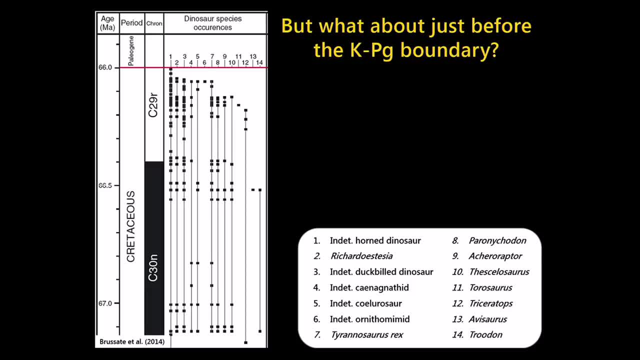 So here on this graph you can see all these dots are either a skeleton or a single dinosaur bone that's identifiable, that's been located in time relative to the extinction event. So if you're interested in knowing what these animals are, I've listed them all here. 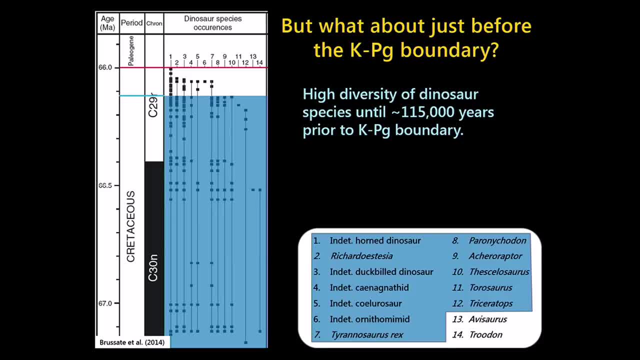 And what you see when you look at that graph is that you can see that up to about 115,000 years before the boundary, you still have a very high diversity of animals. They're all present there. So you have a high diversity dinosaur fauna. 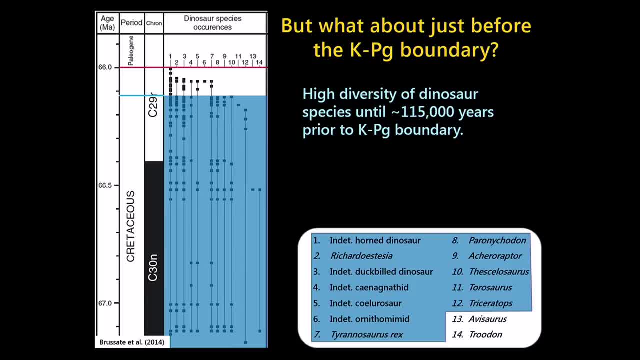 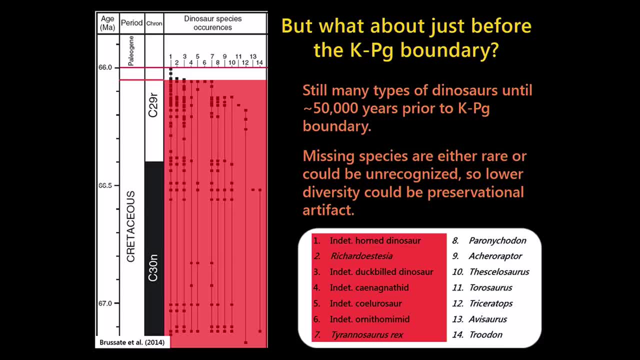 until at least 115,000 years before the boundary. When you get to about 50,000 years before the boundary, then you seem to have some species that have disappeared. But if you look closely you'll see that some of those species 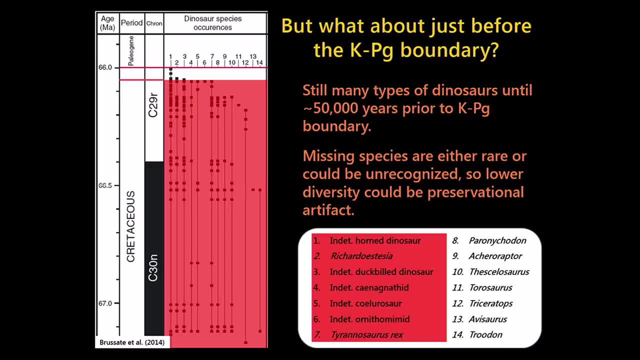 are actually really rare in the fossil record, So it might just be a gap in the fossil record that they're not represented. And then some other species that are missing are actually probably just a matter of identification. So, for example, you see Taurosaurus and Triceratops. 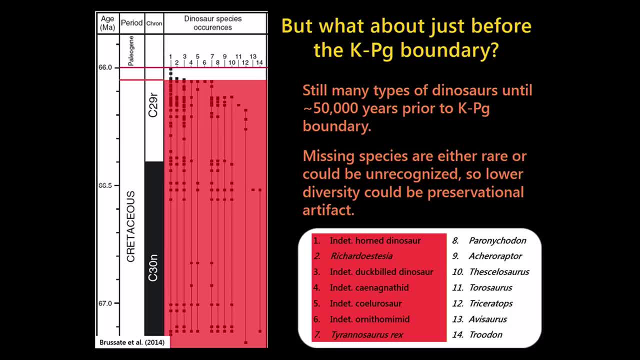 seem to have disappeared, but we still have an indeterminate horned dinosaur's fossils that are discovered. So it means that you know that there's horned dinosaurs around. you just can't identify to which species they belong. So it's quite possible that some of the missing species 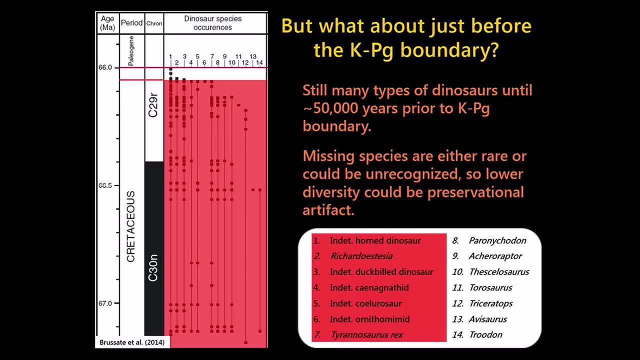 are actually, in fact present, they just haven't been identified. And then, after that, you have a big little gap going on to the boundary, That's the famous three-meter gap. That's a stratigraphic interval where we find very few fossils. 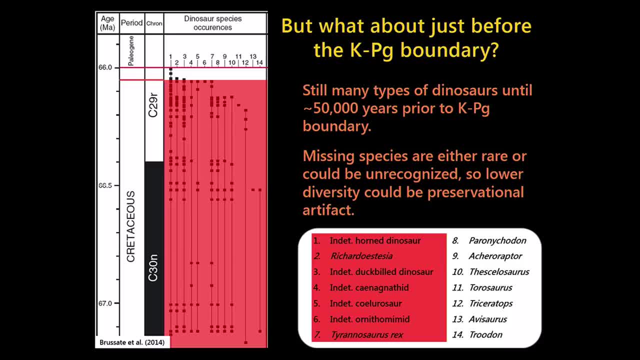 But if you look lower down in sections you can see there's many intervals where we don't find any fossils at all. So it's been argued that that gap here could just be a preservational artifact, not actually an indication that dinosaurs have actually gone extinct. 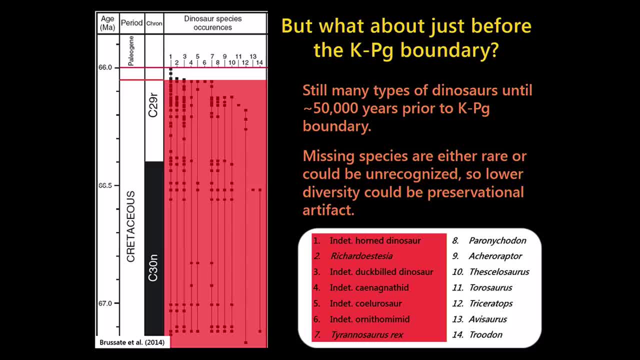 But based on what we see here, we see evidence for high diversity: fauna all the way to at least 115,000 years before the boundary, possibly even closer to 50,000, and maybe even- if you consider that an artifact- possibly all the way up to the boundary. 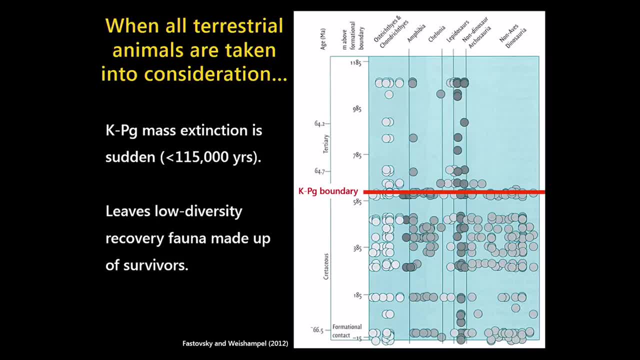 But to be conservative, we'll just assume that dinosaurs went extinct somewhere between the day of the event and 115,000 years before the boundary, And that's pushing the limit of our resolution with the stratigraphic record, So we can say that the dinosaur extinction 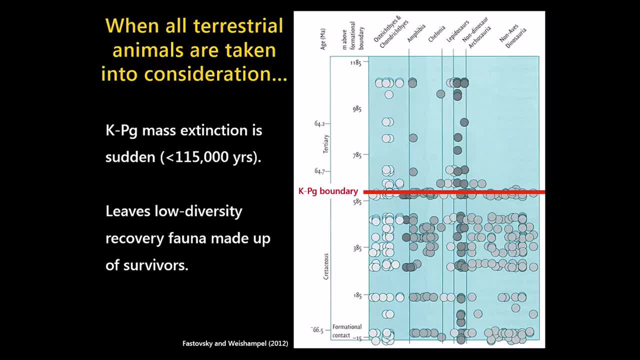 was a sudden event because it happened within a time frame that's hard to resolve using the stratigraphic record. Then if you look at the whole record for including all animals, including some fish, amphibians, crocodiles and dinosaurs- 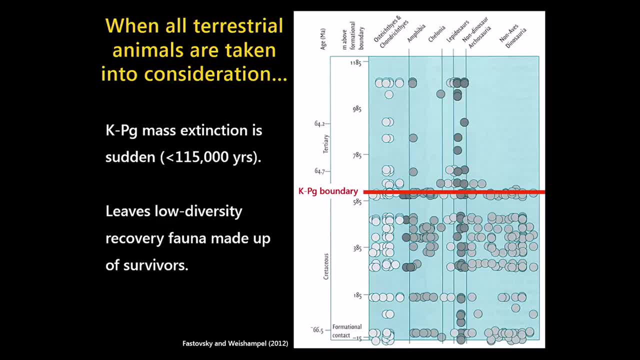 you can see, below the boundary you have a lot of animals being around leading up right to the boundary And then after the boundary you can see you have a much lower diversity, fauna that persists, that consists mainly of the survivors because everything else went extinct at the boundary. 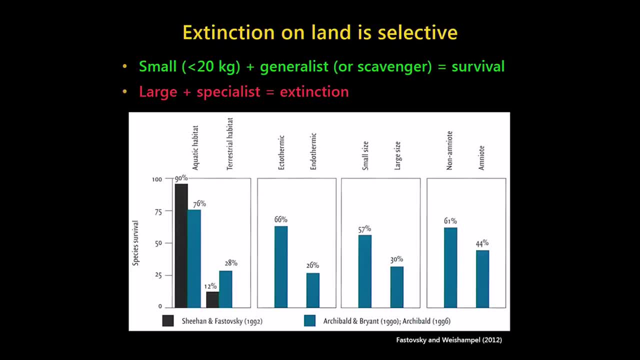 If you look at who survived and who went extinct, you can see that the terrestrial extinction was highly selective. By selective we mean depending on what type of animal you were and what you were doing in an ecosystem that affected your chances of surviving the extinction event. 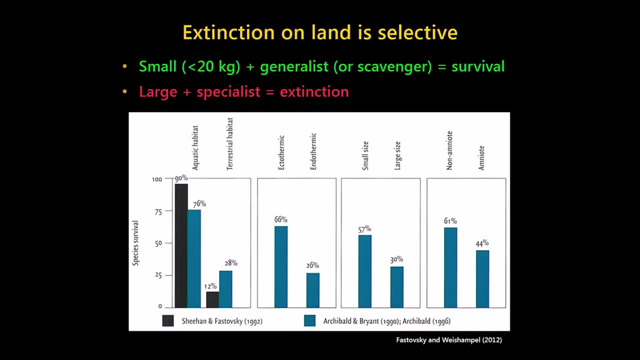 So, for example, if you were an aquatic animal, you were ectothermic or cold-blooded and you were small size. your chances of surviving the event were much higher than if you were a terrestrial animal. you were warm-blooded and were a large size. 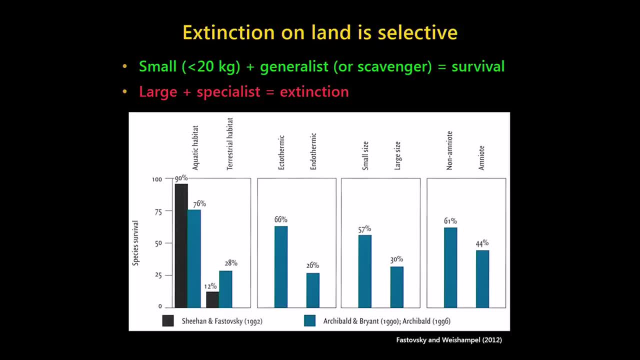 In fact, it's been shown that if you were a small animal, you weighed less than 20 kilos, so that's about 44 pounds, and you were a generalist, meaning that you could eat a little bit of anything or a scavenger. 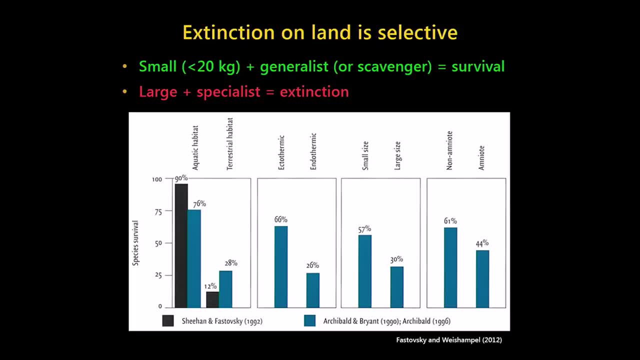 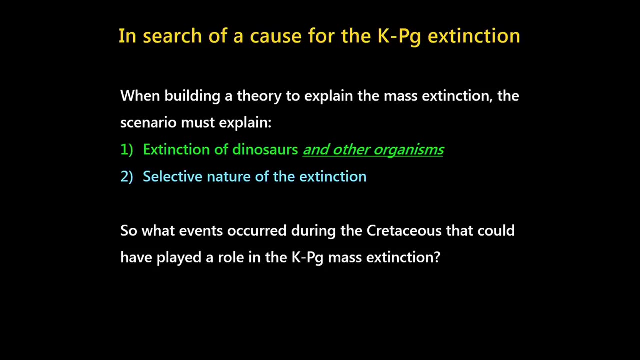 then the chances were that you would survive the boundary event. But in contrast, if you were a large animal and your diet was specialized- you were either a strict meat eater or a strict herbivore- then you were pretty much doomed. So what could have caused the extinction? 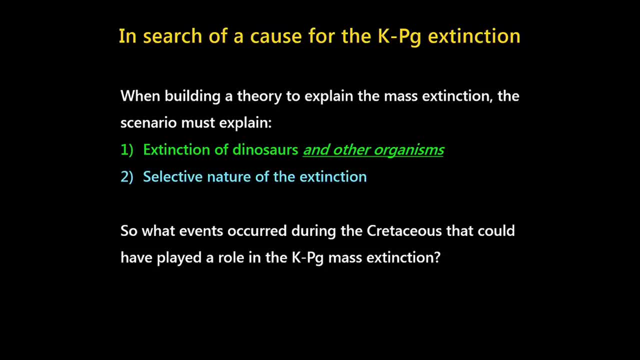 that we see at the K-Pg boundary. Well, when you try to develop a theory to explain the extinction, you have to make sure that your model explains all the lines of evidence at hand. So this means that your model needs to explain why dinosaurs and other animals and plants went extinct. 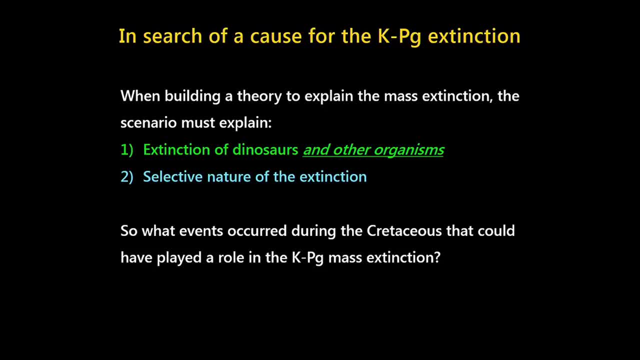 and it also needs to explain the selective nature of the extinction, why some species suffered more than others. So that's why you'll often hear theories thrown out saying: oh yeah, mosquitoes started spreading diseases that killed all the dinosaurs. Well, that doesn't explain why lizards and corals went extinct. 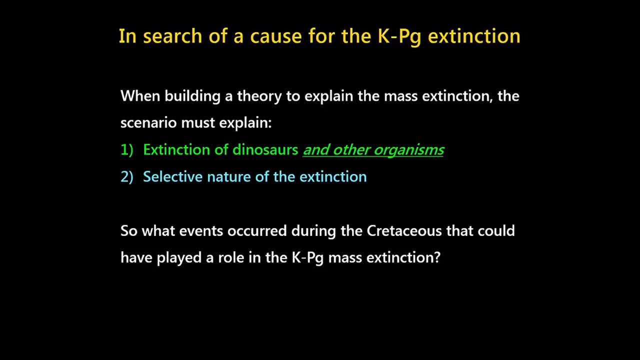 So you have to find a model that actually tries to explain the whole pattern. So we'll now have a look at what events happened during the Cretaceous that could have led, or at least affected the environments and led, to the extinction of all these animals. 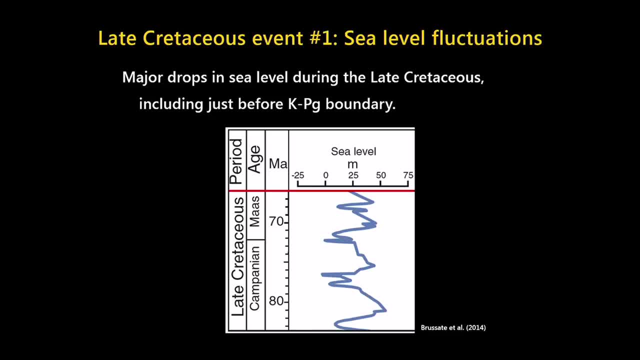 So first, we know that during the late Cretaceous there were major sea-level fluctuations. If you look at the record of sea levels, to the right you have a sea-level rise, To the left you have a sea-level fall. 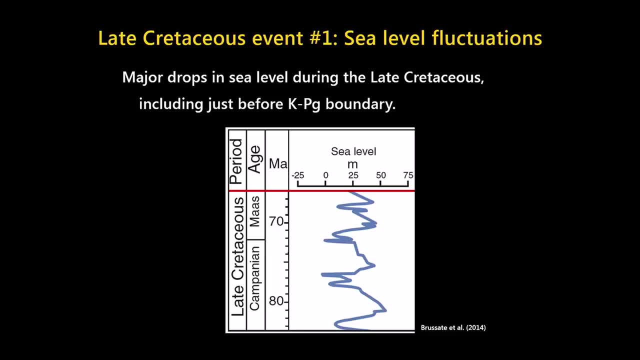 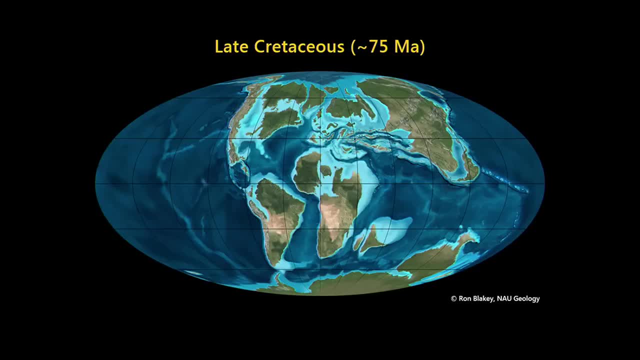 You can see there's lots of fluctuation and just before the boundary we have a last major marine regression or sea-level fall. So if you look at what the world looked like about 9 million years before the extinction of dinosaurs, you can see sea levels are extremely high. 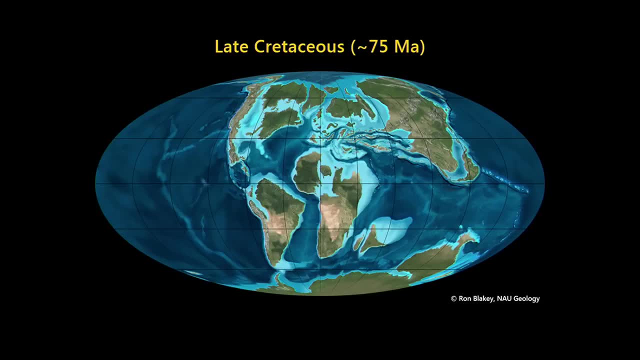 We have large inland seas over North America. Europe is mainly underwater, lots of inland seas in Africa and India. And then, if we fast-forward to 9 million years to the K-Pg boundary, we can see that the sea levels have dropped dramatically. 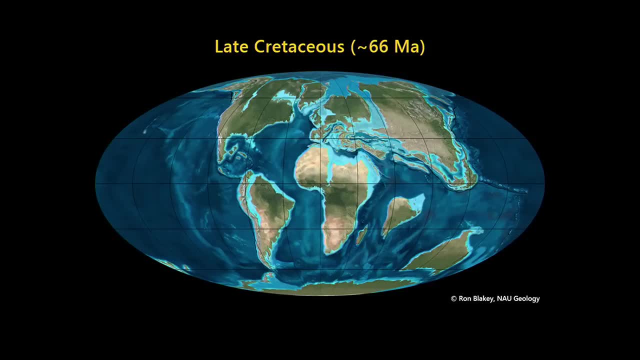 The inland sea is pretty much gone in North America. There's far less water in Europe, Africa and India, So all those marine regressions or sea-level falls could have potentially affected the environments. that would have been a stress to which animals would have needed to cope with. 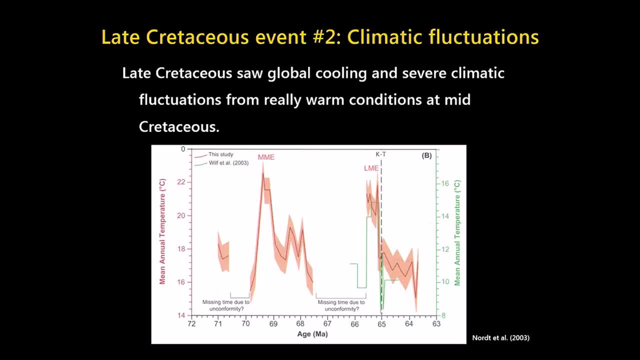 We also know during the late Cretaceous there were major climatic fluctuations. Up to the middle Cretaceous the climate, the world, was usually a very warm place, warm and equable. But when you get to the late Cretaceous, 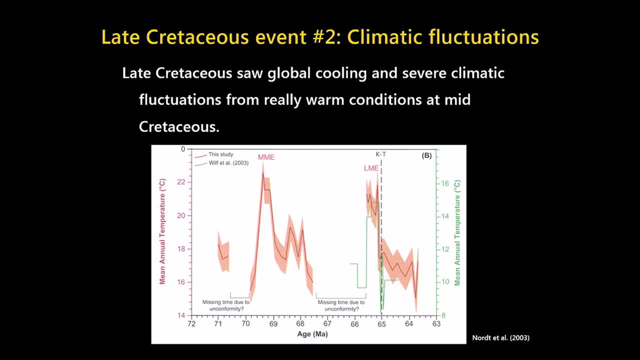 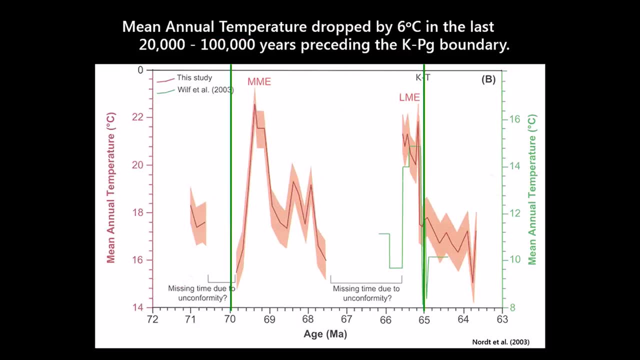 you see a lot of fluctuations, ups and downs. So we have shifts to very warm temperatures, to very cool temperatures And if we look at the last 5 or 6 million years of the Cretaceous and Maastrichtian, we can see that there's lots of. 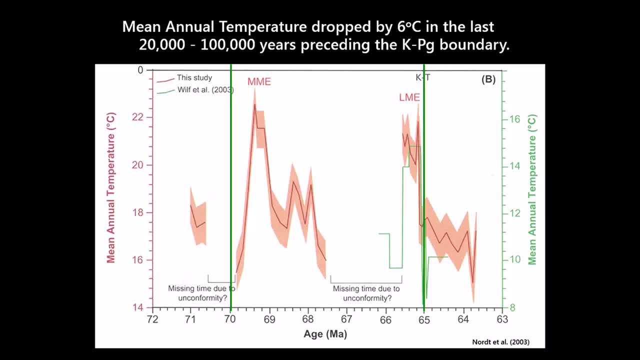 Basically it's a roller coaster ride going to very warm conditions, very cool. And what's really interesting is, just before the boundary, starting about 20,000 to 100,000 years before the boundary, we have a very rapid drop in temperatures. 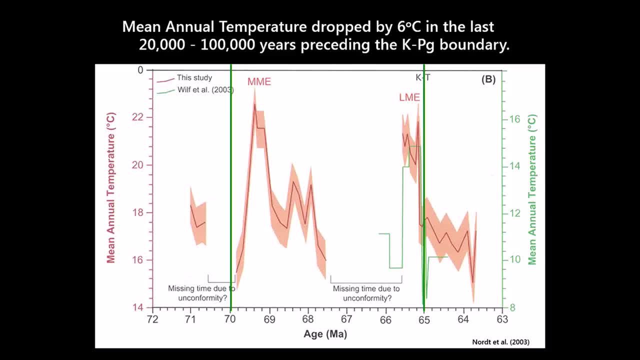 We're talking about a drop in mean annual temperatures of about 6 degrees Celsius. So for Alberta this means we would have gone from a climate similar to what we see in Virginia today, just south of Washington DC, to a climate typical for Minnesota. 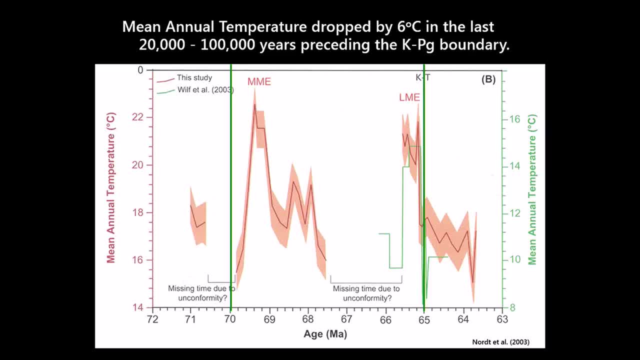 So it would have been a major, dramatic climate shift and that would have happened really rapidly, within 20,000 to 100,000 years. So that would have put a lot of stress on the environments. We also know at the end of the Cretaceous. 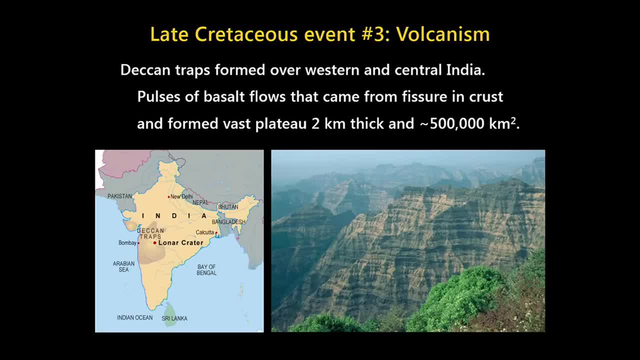 there were major volcanic eruptions. There were eruptions in India. There were big fissures opening up in the crust and large pulses of basalt just started pouring out. and that was almost continuous eruptions. The lava flows just kept piling up on top of one another. 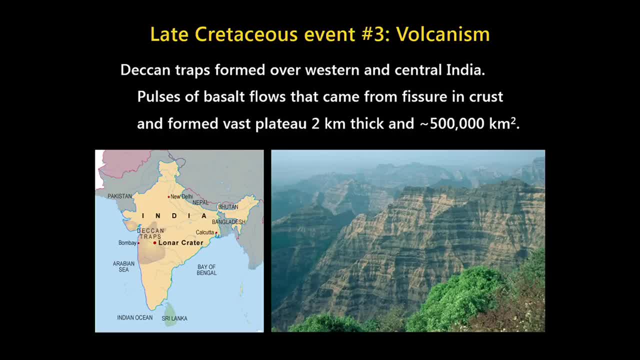 and they formed a plateau that's 2 kilometers thick and around 500,000 square kilometers in area. It's kind of hard to see here, but you can see the Deccan Traps, or the lava flows deposited by the volcanism cover a large part. 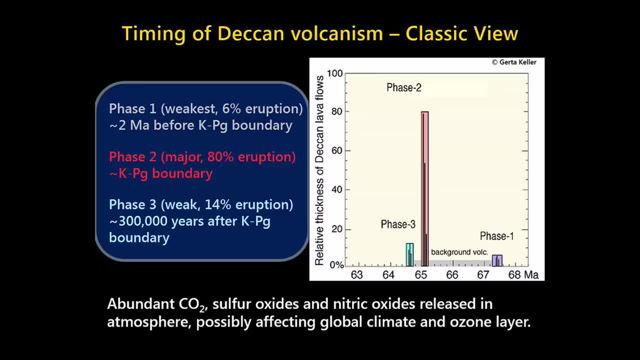 of this Indian subcontinent. So there's a lot of debate about the exact timing of those volcanic eruptions. There's a classic view that presented those eruptions as having occurred over three different time intervals or three different phases. There would have been a very small phase. 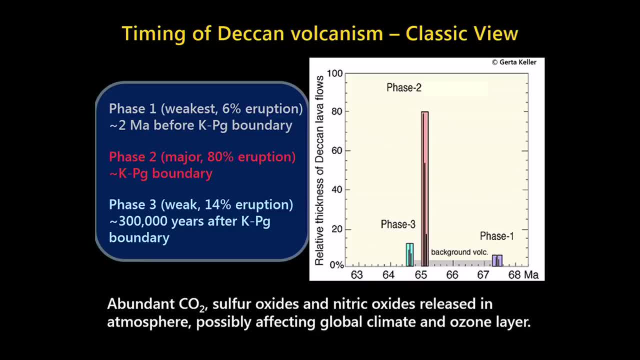 about 2 million years before the K-Pg boundary. A big pulse responsible for 80% of all the volcanic eruptions, right at the time of the K-Pg boundary, and then a little pulse again about 300,000 years after the boundary. 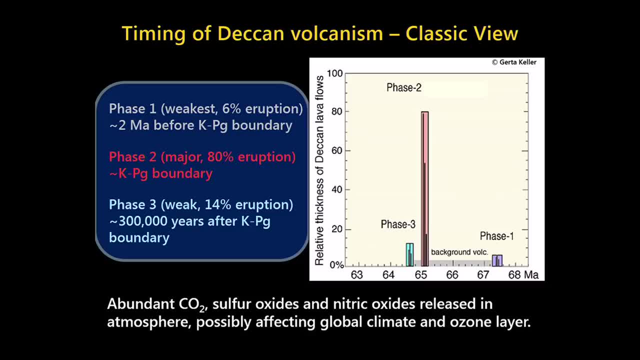 So the proponents of that theory have argued that the volcanism at the boundary would have been so intense that it would have released lots of gases in the atmosphere, could have affected the climate, created lots of pollution and that could have led to, at least contributed to, the extinction. 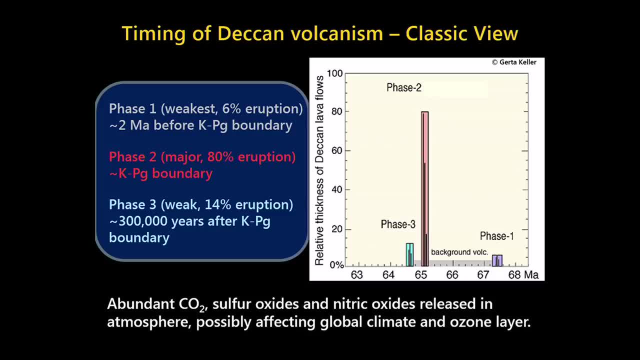 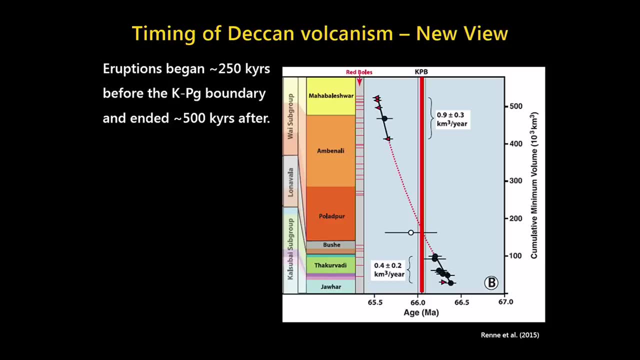 at the K-Pg boundary. However, that view was changed and challenged just last year when a team was able to get radiometric dating, radiometric dates- sorry for samples of the various lava flows of the Deccan Traps, And they've shown that actually. 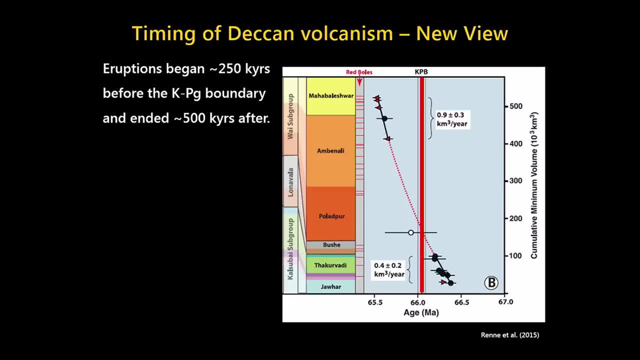 the volcanic eruptions did not occur as three different pulses, but are really concentrated around the K-Pg boundary. What's interesting is that they see that eruptions before the boundary were very frequent, but very small. They're actually responsible for only 30% of the total volume. 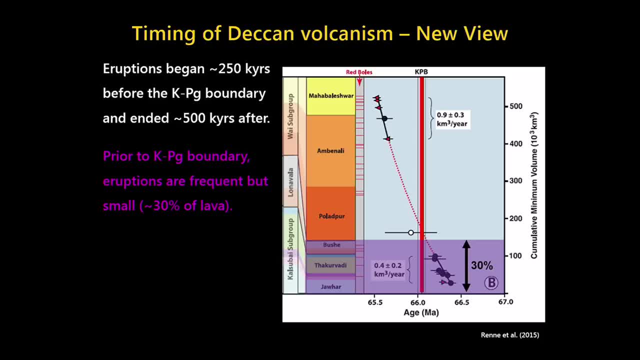 of lava that was extruded. But if you start 50,000 years at the boundary or 50,000 years after the boundary, then the volcanic eruptions become more distant apart, but they're also much more voluminous. They produce a lot more lava. 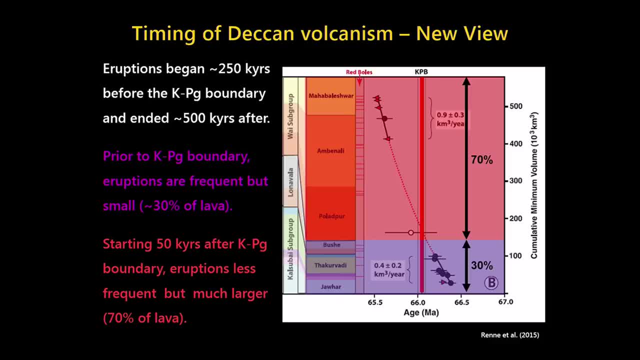 and they're actually responsible for 70% of all the lava flows found in the Deccan Traps. So, following that argument, because the eruptions just before the extinction event, before the boundary, were so minimal, the authors argue that the volcanism. 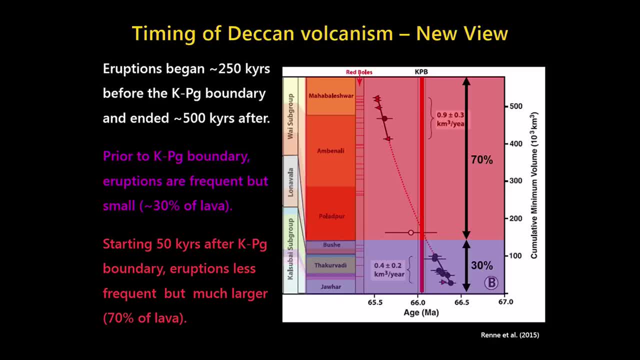 could not have contributed significantly to the extinction event, But the fact that you have a lot of volcanic eruptions after the boundary suggests that it could have actually delayed the recovery, would have had a significant impact on the recovery of animals and probably delayed the recovery. 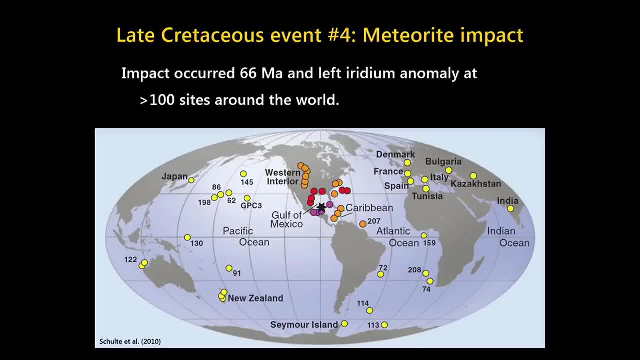 of the ecosystems because there was so much gas released in the atmosphere. Then we're left with a fourth event at the end of the Cretaceous and that's a major meteorite impact. We know that was an impact at the end of the Cretaceous. 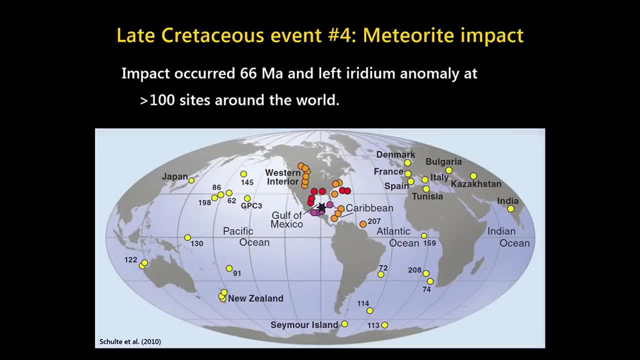 because we find iridium at over 100 sites all around the world. Iridium is an element that's really rare at the surface of the Earth, but it's really common inside the Earth and in meteorites. So how do we know that it's actually? 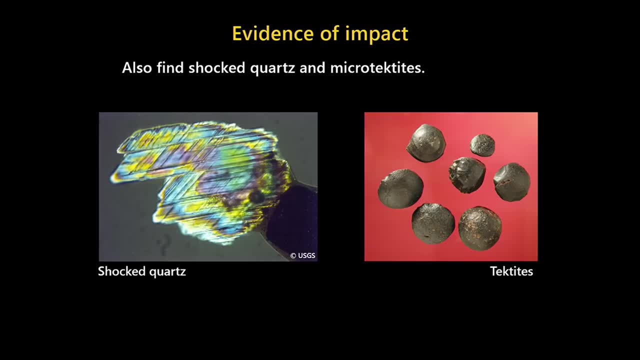 coming from meteorites and not coming from inside the Earth through volcanic eruptions. Well, it's because we find other lines of evidence saying that there was a meteorite impact. We find shucked quartz, which are grains of quartz that are fractured in that. 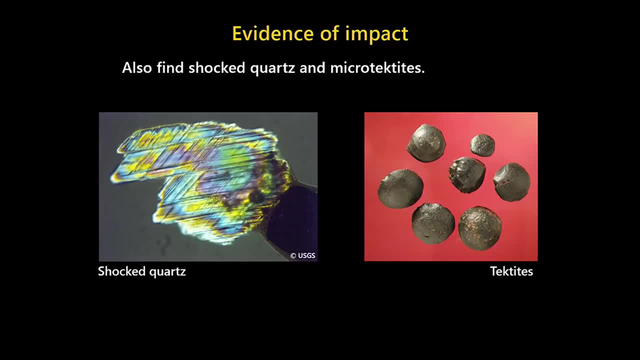 crosshatch pattern indicating that it's been subjected to intense heat and pressure, typical of what you see in impact sites. And then we also find tektites. Those are beads of molten rock that have actually fallen down from the sky after having been. 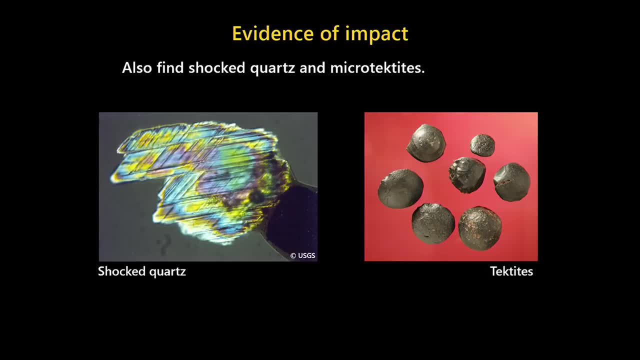 ejected out of the crater, out of the impact site. So the fact that we find all three together- the iridium, the quartz and the tektites- indicates that all that was due to a meteorite impact. But where is the crater? 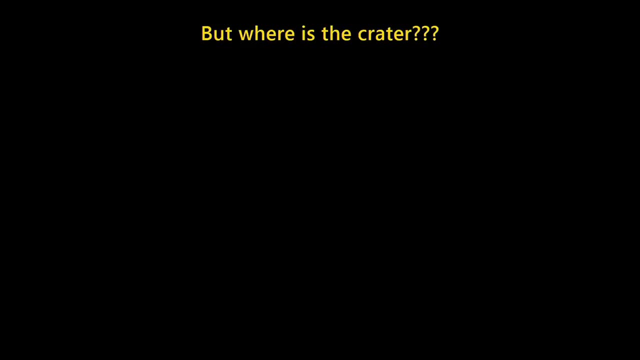 That was the big question. after people found evidence of the impact, They couldn't find a crater. There was no crater that they could find that was right at the K-Pg boundary. So there were different theories. Maybe the crater was gone. it had been totally eroded. 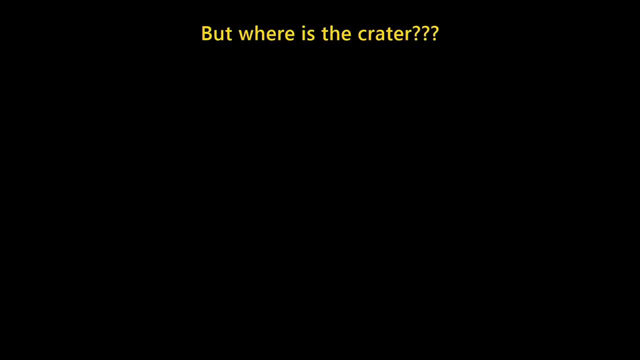 or it had been destroyed in a subduction zone, so the crust would have sank under a continent and nowhere to be seen, Or the crater was actually buried somewhere and just needed to be found, And that's what actually happened As early as the 1950s. 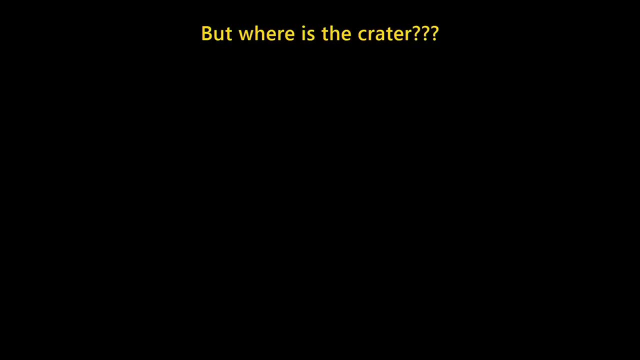 Mexican oil companies were surveying the Gulf of Mexico looking for oil reserves and they came across a large anomaly that they thought could be a crater. but they kept it secret for the longest time And it wasn't until the 80s when geologists heard about the rumors. 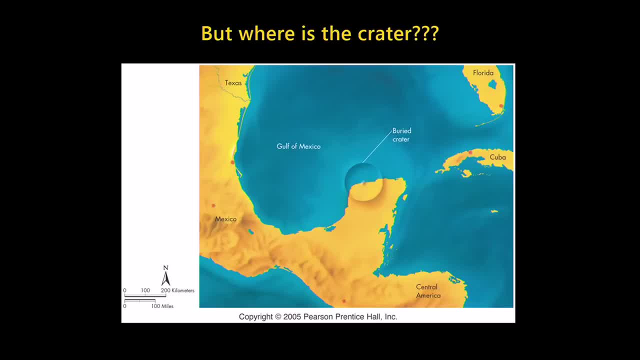 and were able to get their hands on the data, that they discovered that, yes, indeed, the crater was buried under the Gulf of Mexico. The crater is actually halfway under the Gulf of Mexico and halfway under the Yucatan Peninsula And the epicenter, or the center. 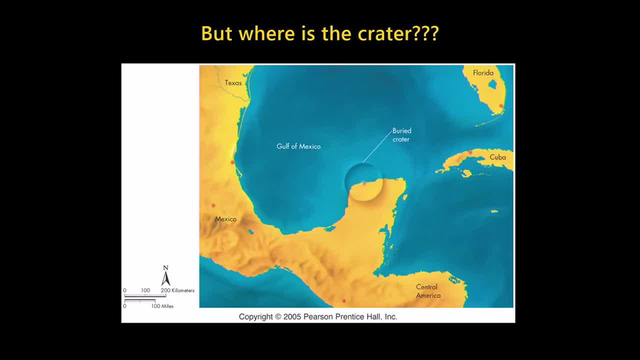 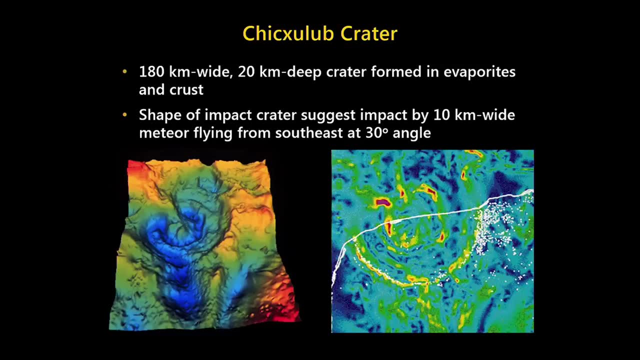 of the crater is close to the town of Chicxulub, So they called it the Chicxulub crater. Now the crater is hidden underground. It's been filled by millions of years of sediment so you can't see it. 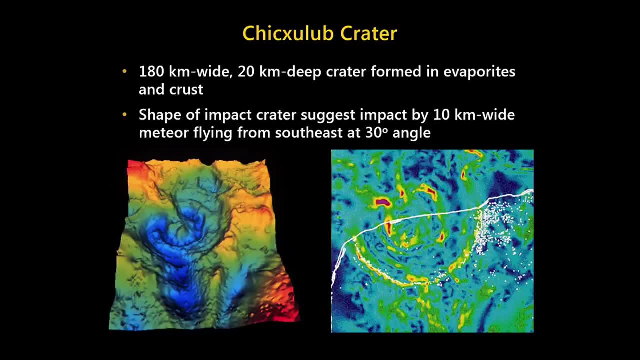 But using geophysical data or techniques, you can actually document its shape and its size. So geologists, using those data, were able to see that they're dealing with a 180 kilometer wide crater, up to 20 kilometers deep, and it formed. 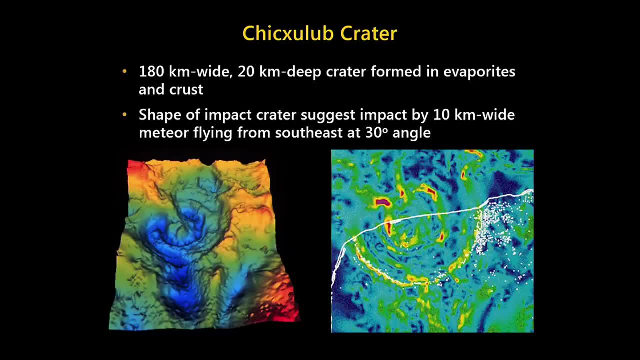 and evaporates in the continental crust right at the KPG boundary. So here you can see that's the raw geophysical data Here. this is a 3D rendering of the crater. You can see it's not symmetrical. You can see there's a big circle there. 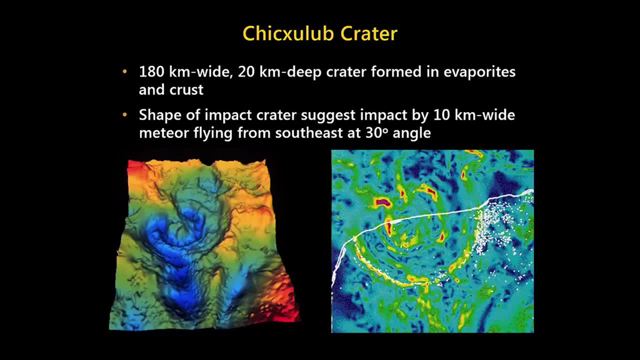 but there's a trough also to the south And, based on the shape and the size of the crater, they were able to say that the crater was produced by a meteorite that was 10 kilometers in diameter and it came at a shallow angle from. 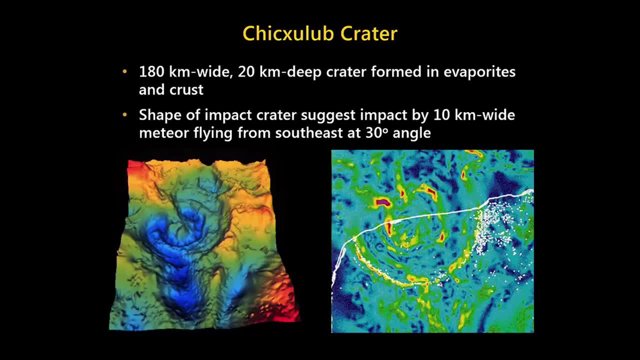 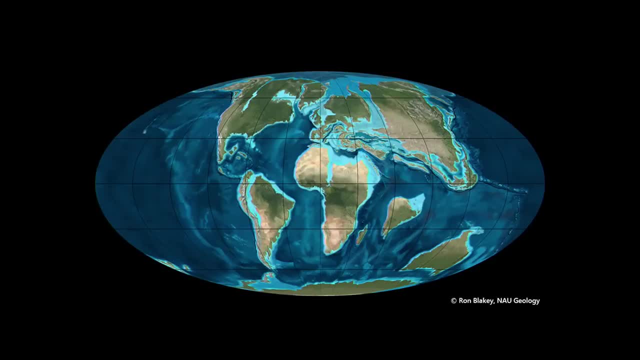 the southeast. So it wasn't a dead-on collision, It was basically more of a glancing blow at 30 degrees angle relative to the surface of the Earth. So if we look at what the Earth looked like 66 million years ago at the KPG boundary, we can imagine. 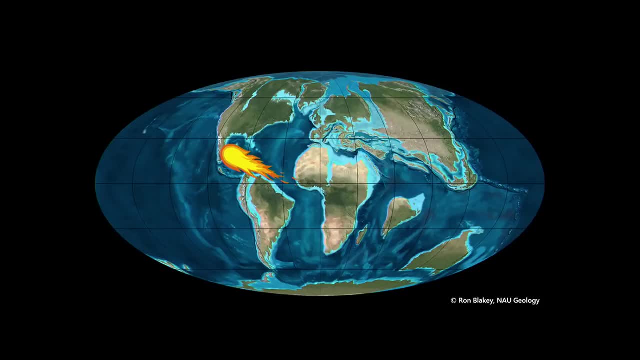 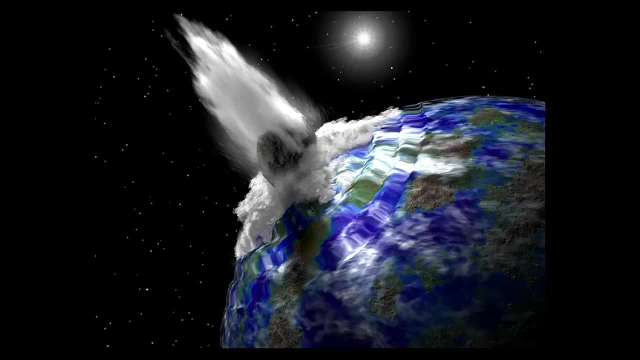 the impact coming in and colliding, crashing in the Gulf of Mexico right there. So lots of reconstructions are very dramatic. They show that head-on collision, a meteorite cramming into the Earth. But those reconstructions are wrong. It's definitely. 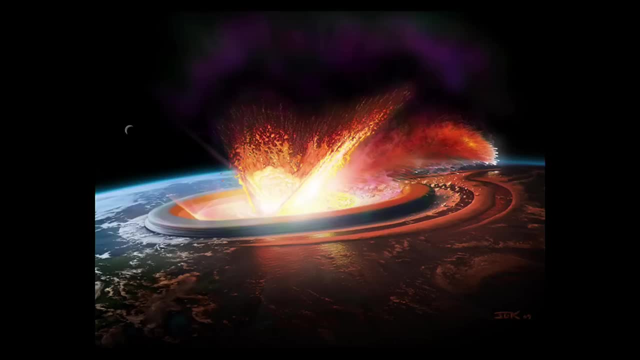 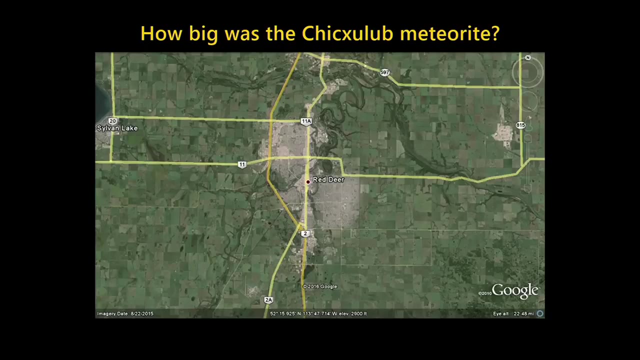 more of a glancing blow. The meteorite came at a very shallow angle and just scraped the surface of the Earth and just crashed there. So telling you dimensions like a 10 kilometer wide bolide or meteorite and a 180 kilometer wide crater. that can be. 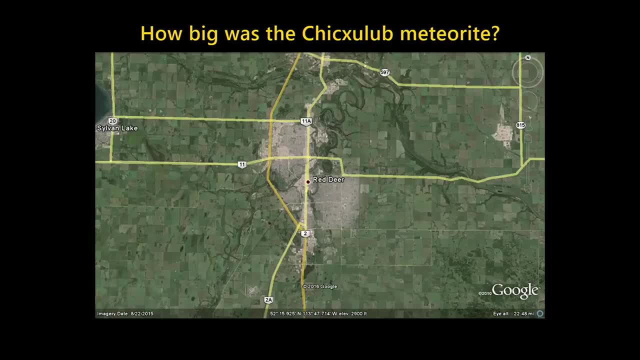 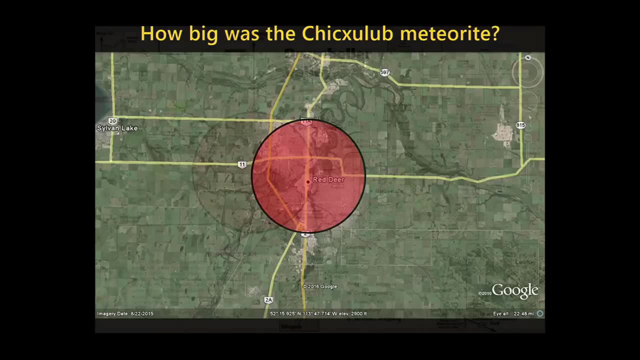 hard to understand, So I decided to plot those dimensions on things that are familiar to us. So if you want to think of a 10 kilometer wide meteor, you're talking about a chunk of rock the size of the city of Red Deer. 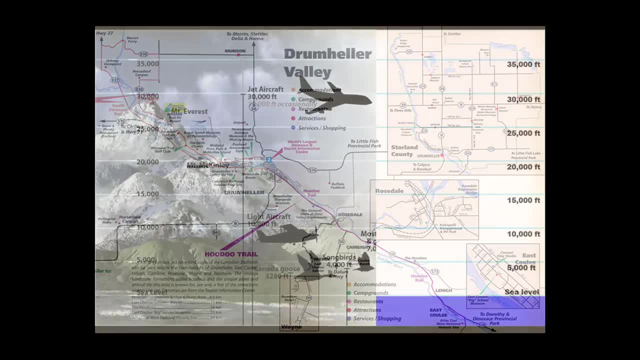 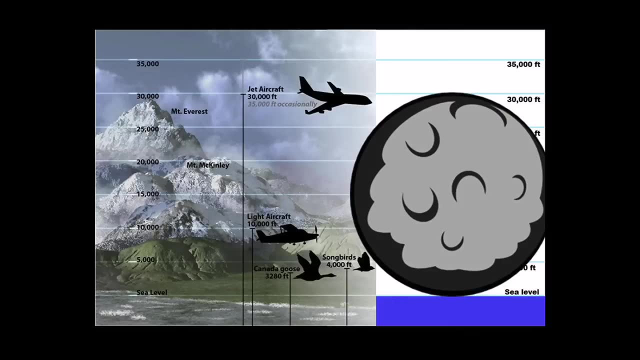 Or if you were to lay down, if you were to sit at sea level, the other end would actually be higher than the Everest and would actually reach the cruising altitude of most major commercial planes. So it's a very large chunk of rock that hit the Earth. 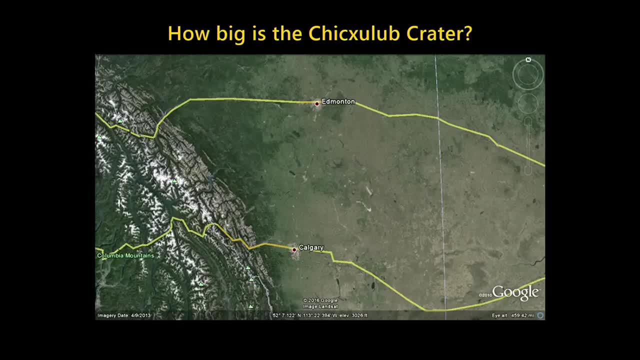 And if you think of a 180 kilometer wide crater and you set it over central Alberta, it would go from Calgary all the way to Ponoka, about 50 kilometers north of Red Deer, And then you have to think that that hole is. 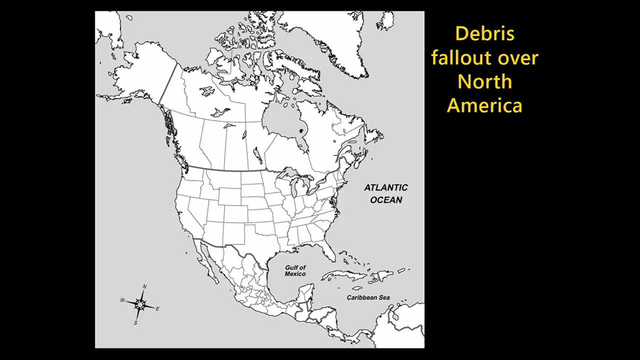 20 kilometers deep, So it's a very, very large crater. So, of course, with a collision coming from the southeast at a very low angle, that collision just catapulted a lot of debris out in the air and just ejected lots of debris. basically just 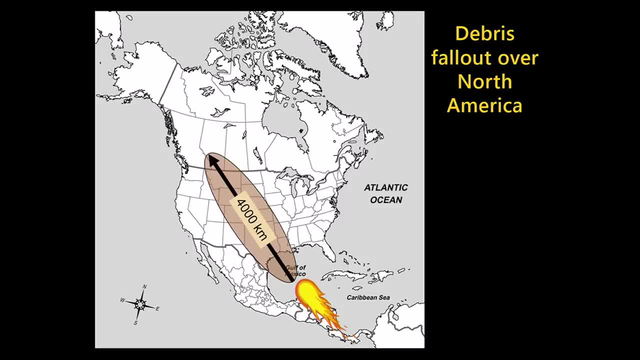 spraying all over North America, such that we find debris, direct debris fallout, as far north as central Alberta, here 4,000 kilometers away from the crater. And even today we still find several sites over the western interior where we have actually that boundary, that impact. 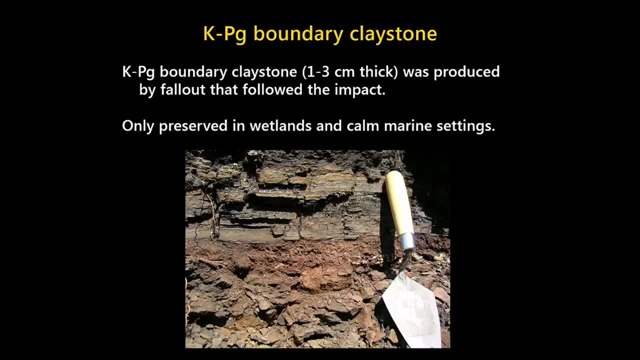 that debris from the impact preserved. That's what we call the KPG boundary claystone. It's a brownish salmon colored mudstone that's about three centimeters thick and it is the record of the direct impact of a meteorite 66 million years ago. 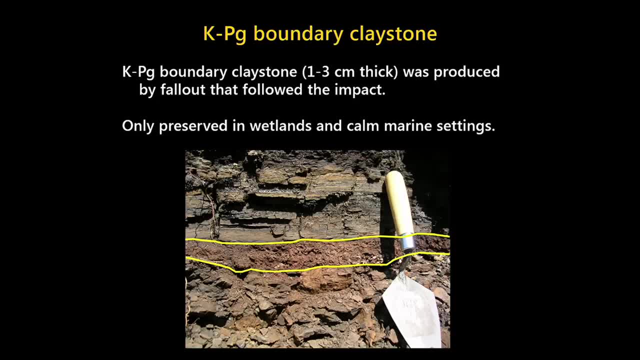 That boundary claystone is usually preserved at the base of coal beds, so they formed in swamps and they're also found in calm marine settings. We need very calm environments to preserve that boundary claystone so that it can gently settle down to the bottom and be buried. 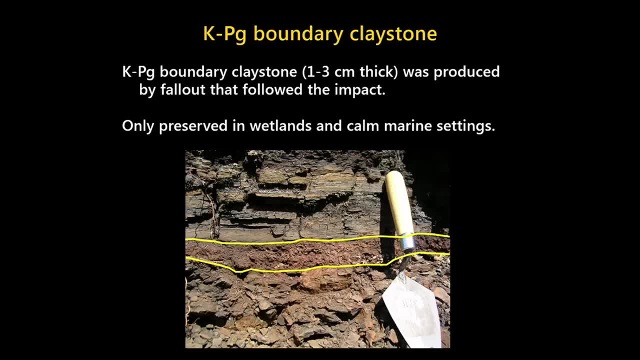 without disturbance, That layer of rock would have been deposited on the flood terrain and everywhere, but rain, wind and whatever would have actually reworked that debris and just scattered it around. So that's why we find it preserved only in very calm settings. 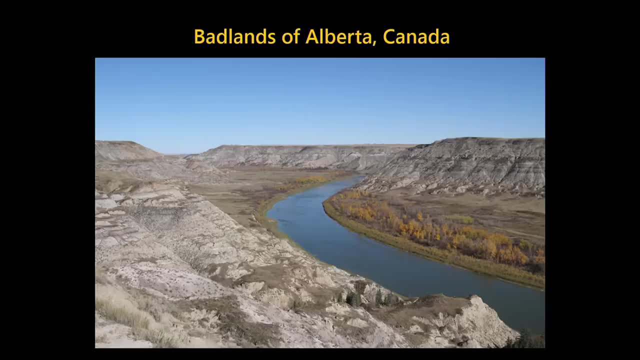 So one of the best sections and most extensively studied sections is actually located just north of Drumheller, about an hour north of here, close to the town of Huxley. It's been extensively studied by the likes of Dennis Braman from the museum Art Sweet, from. 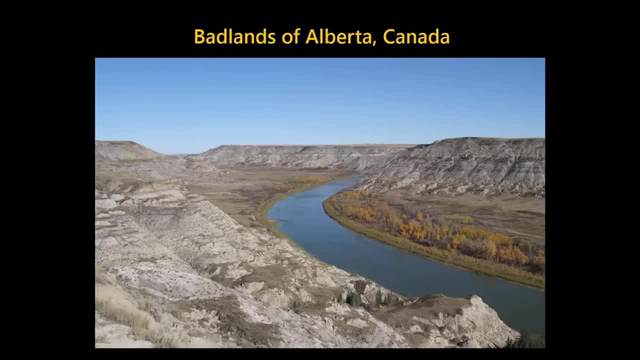 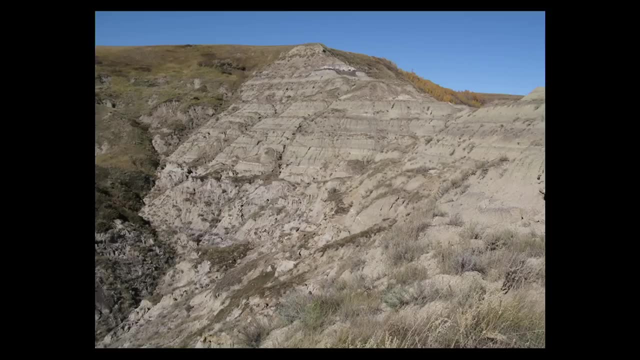 the GSC, and myself and colleagues here have also contributed a little bit by studying the isotopes across the boundary. So we know a lot on that section and actually it can be really helpful to help us reconstruct the aftermath of the impact. So here we have a nice photo. 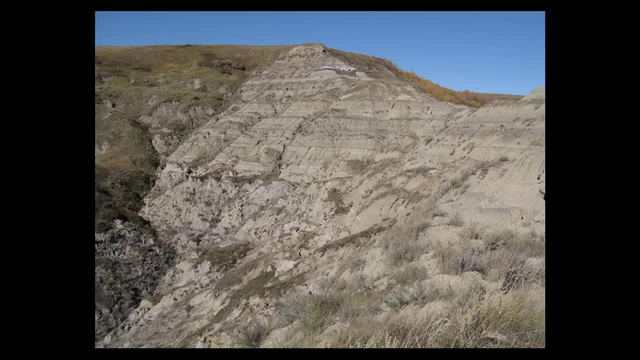 showing what the outcrops at Knudsen's Farm look like. We have a rock record that represents the last million year or so of the age of dinosaurs, and the KPG boundary can be found near the top of the outcrops at the base. 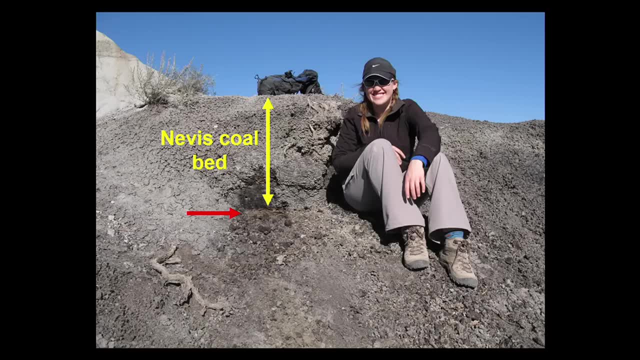 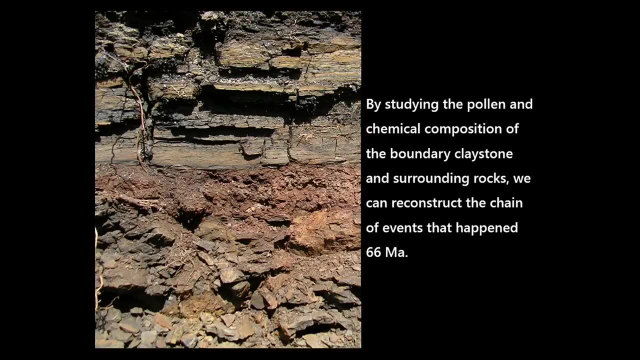 of the coal bed. We have about a 45 cm thick coal bed and right at the base you have that nice little brownish mudstone, the boundary claystone. So you can see it here at the overlying mudstone and just at the 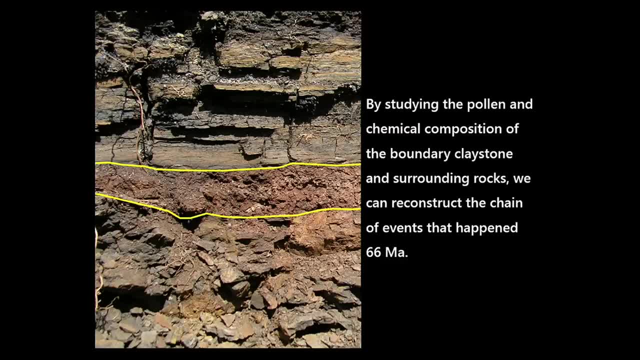 base of the coal And by studying the pollen and the chemistry of the rocks surrounding the boundary claystone and the claystone itself, you can actually reconstruct the sequence of events, the environmental changes that happened before the impact, during the and afterwards. So what I'll do now is actually show. 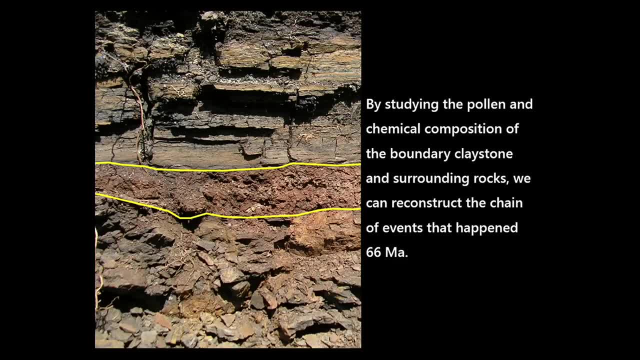 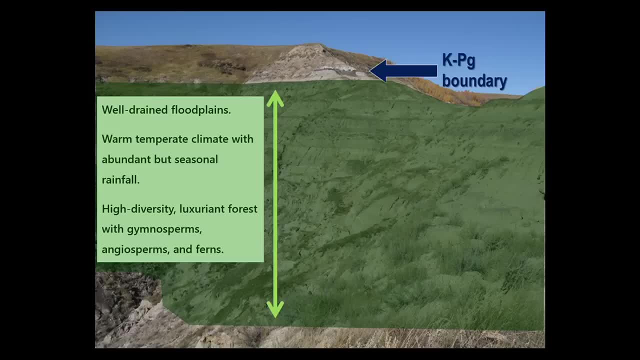 you what the record says, what happened during the Cretaceous and what were the consequences of the impact. So if we start by looking at the section overall, you can see from the base of the section up to about 3 meters below the boundary claystone. 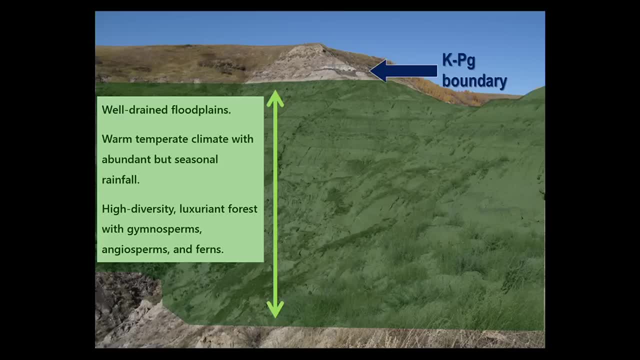 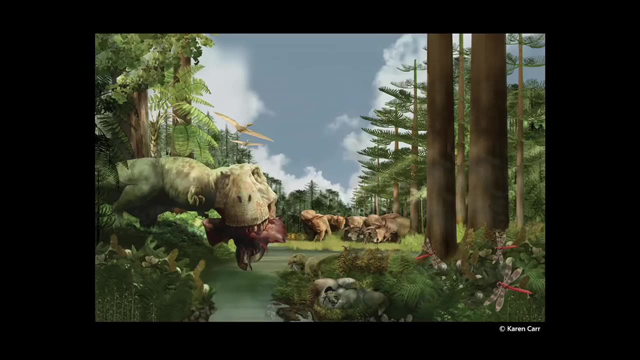 we have evidence of very well drained habitats, very well drained floodplains, we have a warm temperate climate, lots of plants with abundant but seasonal rainfall, and then we have a very high diversity of variant forests dominated by different plants. So here's a reconstruction of what the 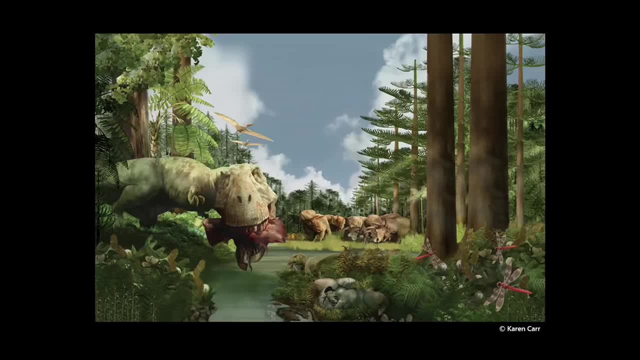 landscape could have looked like at the beginning of the end, so to speak. So you can see that forests are dominated by large gymnosperms or conifers, evergreens. The understory was mainly composed of angiosperms or flowering plants. They were not forming the trees. 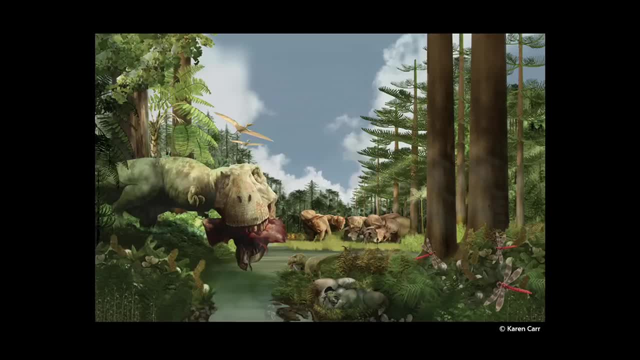 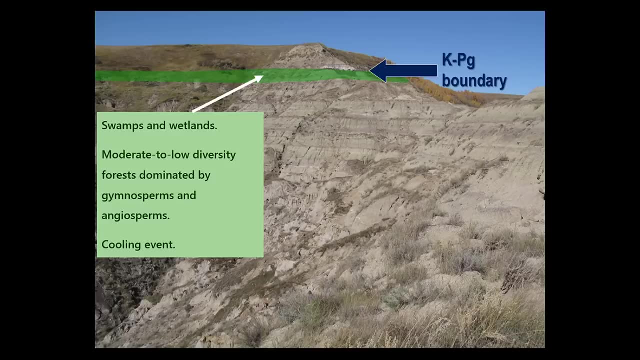 they were the understory. And then you also have lots of ferns around. Then, starting 3 meters below the boundary claystone up to the boundary claystone, we have an environmental change. We see a shift to wetland conditions, So the water table is rising. 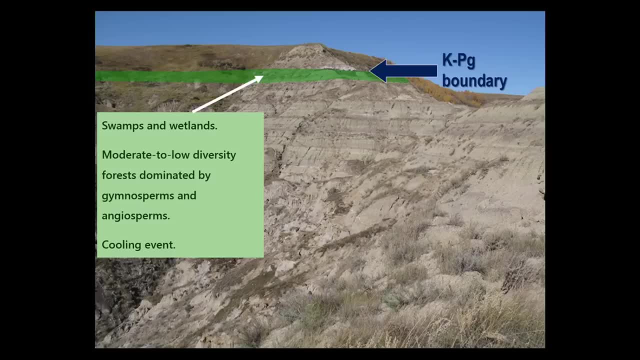 forming more of a swamp. We have a slight decrease in diversity of plants, so we have a moderate to low diversity forest. now, And that's probably the interval where we see the cooling event that I mentioned earlier: the onset of a drop of 6 degrees Celsius. 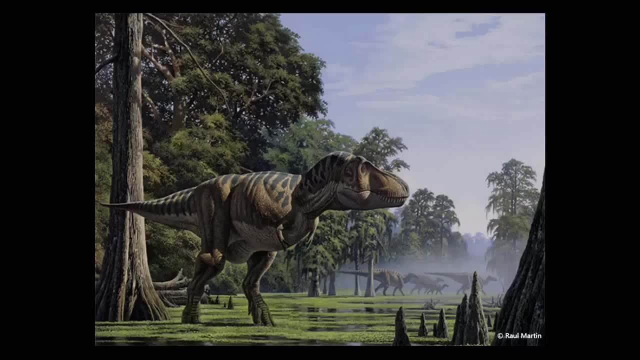 in the mean annual temperatures during that interval. So that is what the environment would have looked like. You can see it's much wetter, there's swamps, but the dinosaurs are still happy and walking around. Then we look closely at what happened. 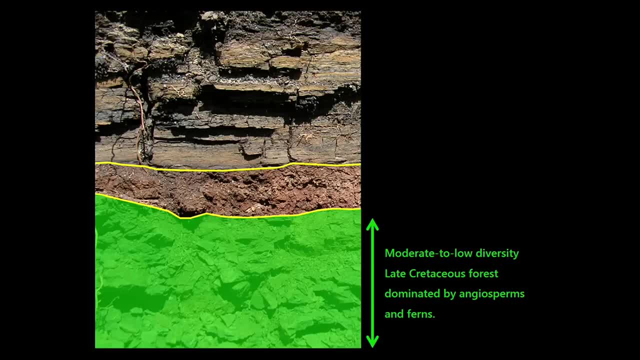 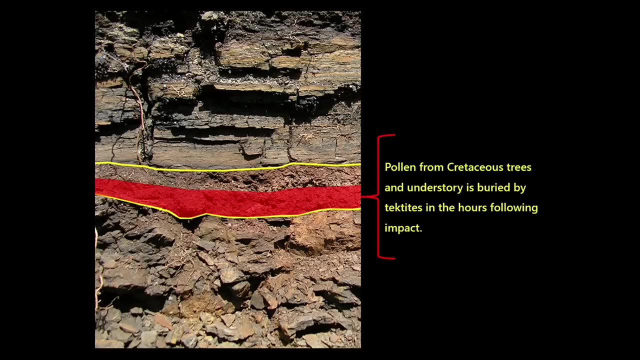 just before the boundary, So just below the boundary, just before the impact, we have that typical forest: slightly lower diversity, but lots of plants growing around, And then, the day of the impact, we have that layer of rock that gets deposited. 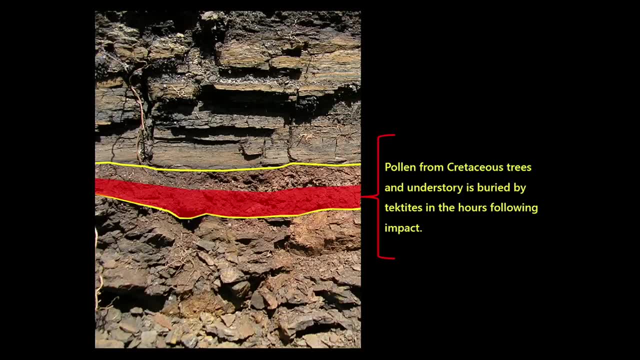 And it preserves actually pollen from Cretaceous trees that are just being buried by the tektites falling from the sky. So the impact happened in Yucatan: projected a lot of molten rock up in the atmosphere and, as it cools down. 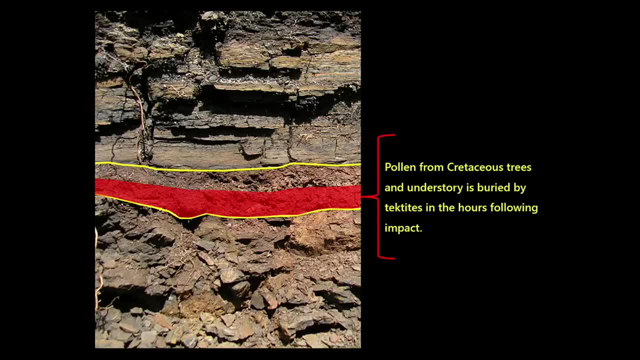 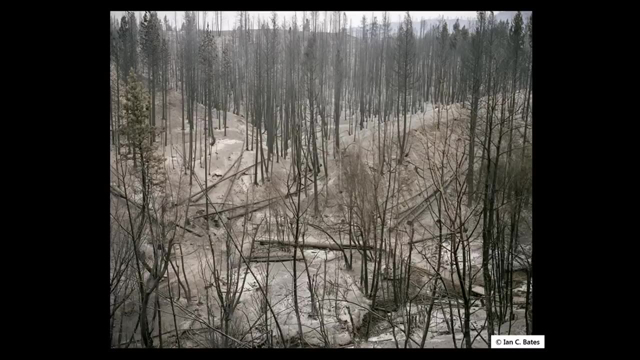 it forms those beads that are just falling down and raining down on the sky covering the landscape. Those beads are still warm, so they probably generated forest fires and the entire landscape, burying all the plants that were present. So here's a little photo illustrating. 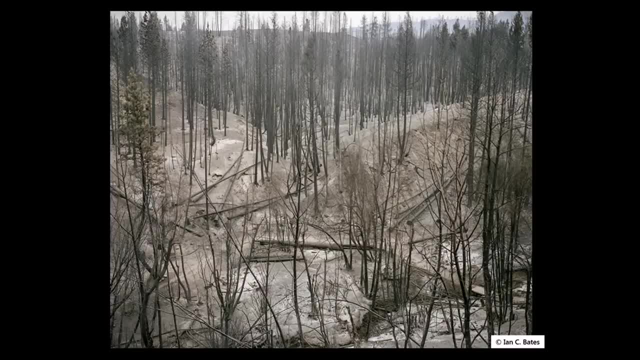 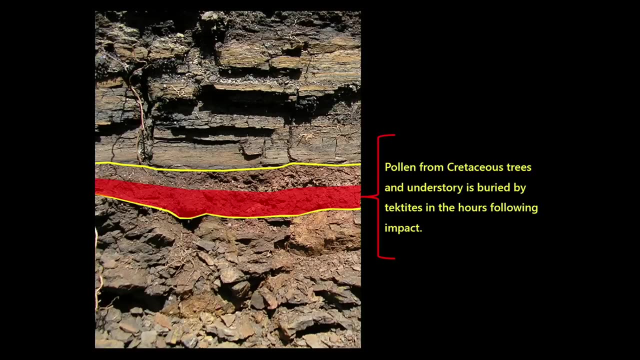 what that day would have looked like. You can see, the entire landscape is just devastated. All the plants are dead, the trees have burned down and the entire landscape is covered by debris falling down from the atmosphere. And that would have happened. that layer right here. 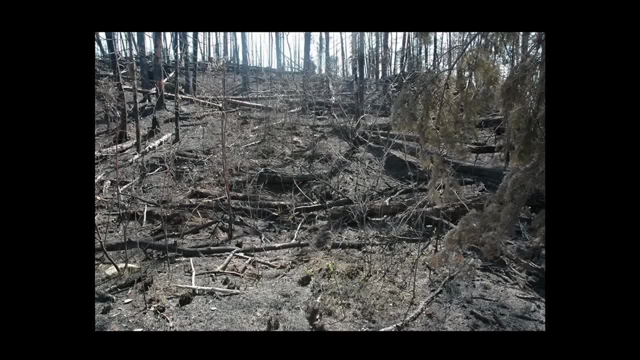 would have been deposited in a matter of hours. because of the debris and then the understory: all the plants are dying and their pollen is just being buried under the tektites that now cover the ground. So if we look at the upper part, 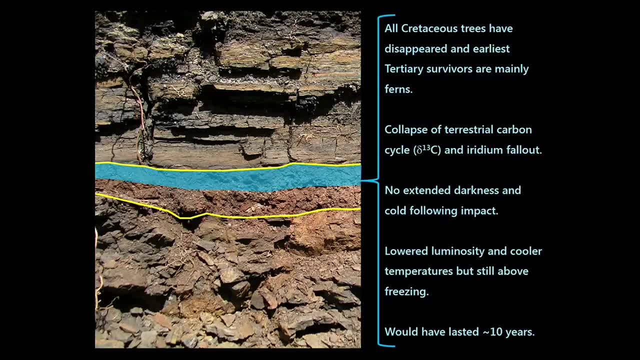 of the boundary claystone. now we can see that all the Cretaceous plants have gone, extinct. The only things that survived during that time interval are ferns that are growing on the landscape. Nearly all other plants are gone. Based on the carbon-13 isotopes. 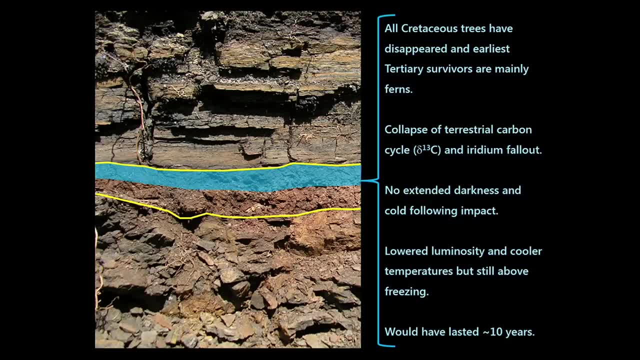 we see there's a collapse and everything shuts down. We also have iridium falling out of the sky. That fine dust that stayed in suspension is slowly settling down on the ground, forming the iridium anomaly. We don't see any evidence. 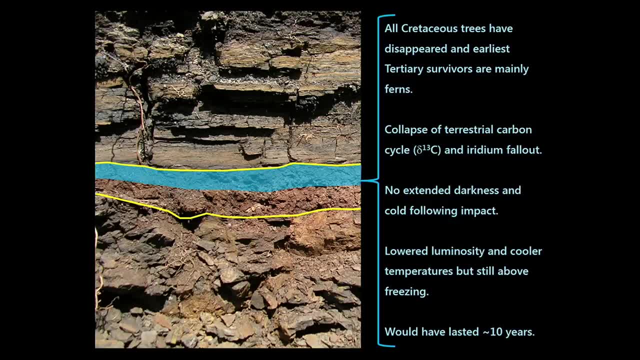 of a nuclear winter. so there's no basically eternal darkness and snow covering the ground, But we do see a decrease in light and a decrease in temperatures for a little while after the impact, and that's probably due to a shroud of dust. 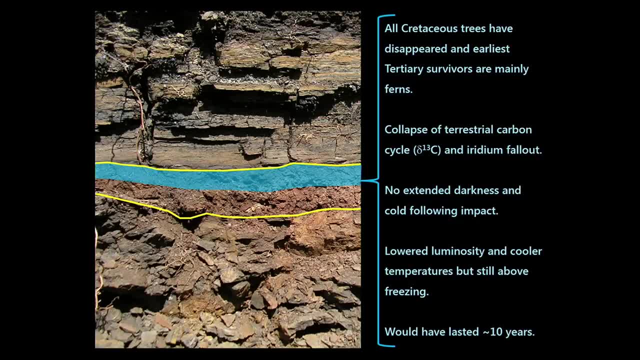 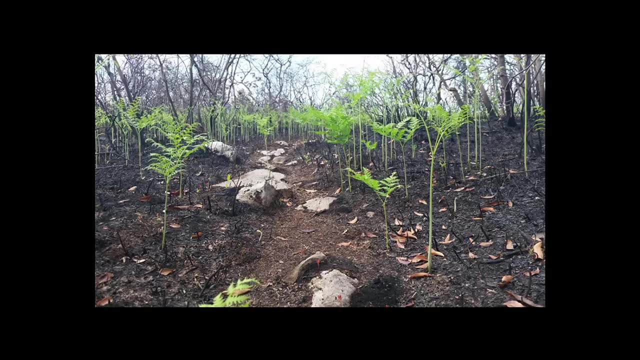 that's still high up in the atmosphere that's blocking the sun rays. And then that period here, based on the laminations that you preserve in that upper part of the boundary, claystone, could have lasted about 10 years. So here's what the landscape would have looked like. 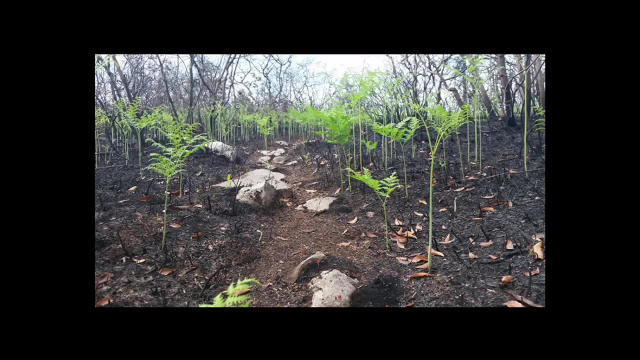 after year one, All the plants are dead, but the only things that managed to regrow are the ferns, And ferns are early colonizers. Even today, after a forest fire, ferns are the first ones to return. That's probably what the landscape 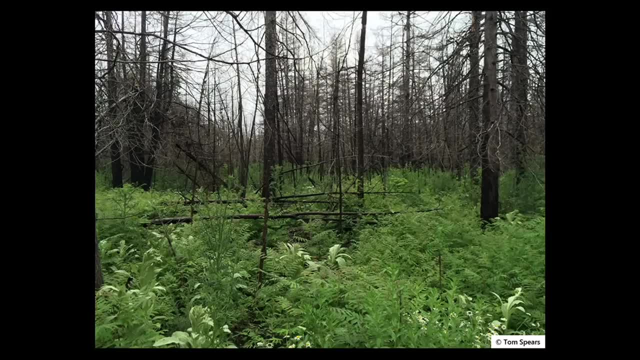 would have looked like, And after 10 years that's what it would have been like. You can see the trees are all dead, but you have fresh regrowth in the understory, Lots of ferns, but you also have a few angiosperms. 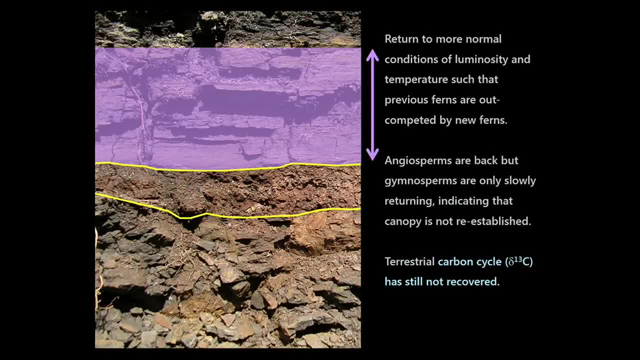 or flowering plants around. Then we go up above the boundary claystone, We have the onset of deposition of coal, so it's a swamp. You have lots of organic matter washing into the swamp And there you have a return to more normal plants. 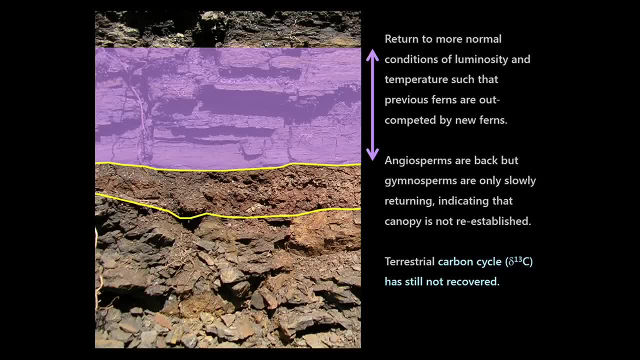 The flowering plants are slowly returning, but the gymnosperms, the evergreens, are still away. So this means your forest doesn't have a canopy. basically, You don't have the big trees, you just have small brushes and bushes that are growing close to the ground. 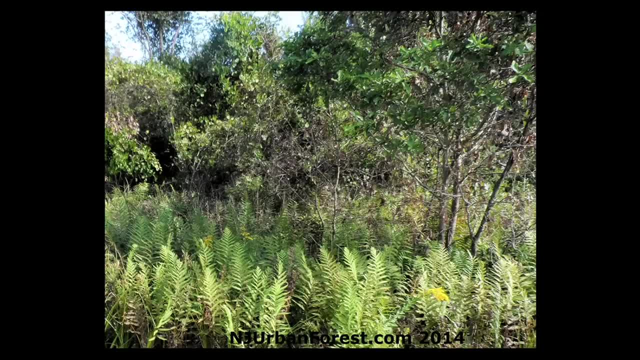 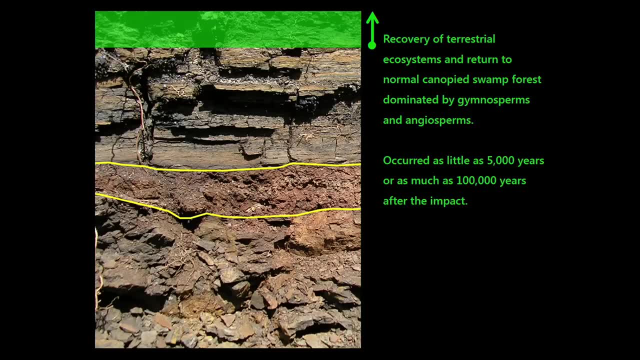 but the terrestrial carbon cycle is still not back to normal, So it's telling you that you still don't have a healthy ecosystem. yet You have basically lots of ferns growing on the ground, so, starting about ten centimeters above the boundary, claystone. 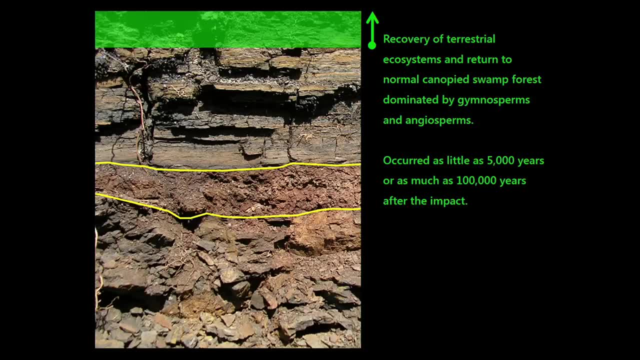 we start seeing a full recovery of the terrestrial ecosystem. So the trees are back. We have a luxuriant forest dominated by gymnosperms. The angiosperms form the understory, And that return to normal could have occurred as soon as 5,000 years. 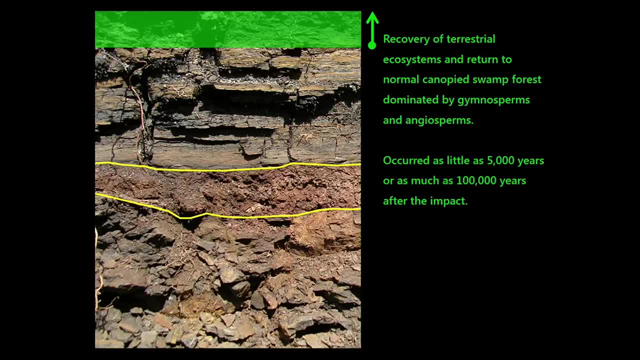 after the boundary, or as much as 100,000 years after the boundary. But now there seems to be mounting evidence that that actually occurred closer to 5,000 years after the boundary, So it would have been a relatively quick recovery. So here's what the landscape 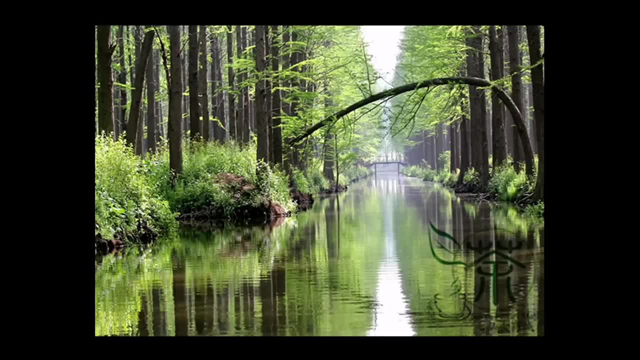 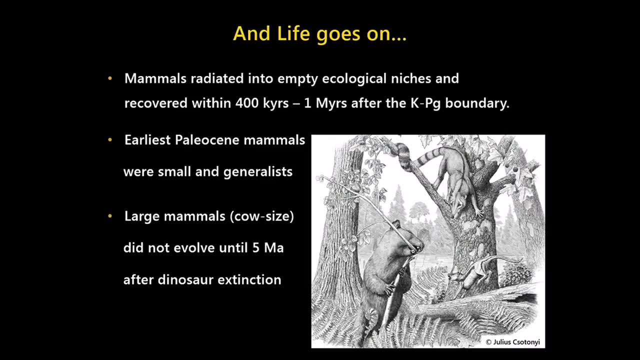 would have looked like at the end of the Cretaceous. You can see all the forests, the trees are back, dominated by gymnosperms, and the understory is mainly angiosperms or flowering plants, And then afterwards we have the recovery. 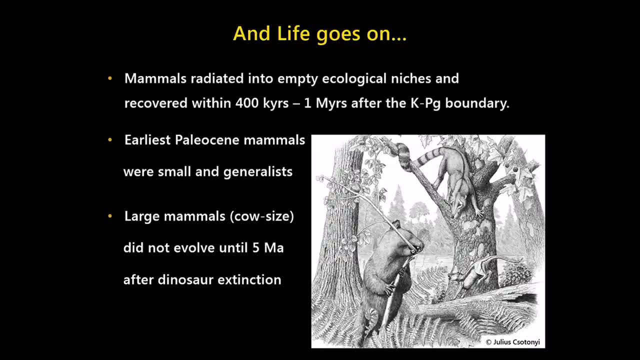 of the fauna. So the animals come back. mammals radiated in the empty ecological spaces left by dinosaurs, but it took them a while. For a while they stayed at very low diversity, but now we have mounting evidence that the mammal ecosystem 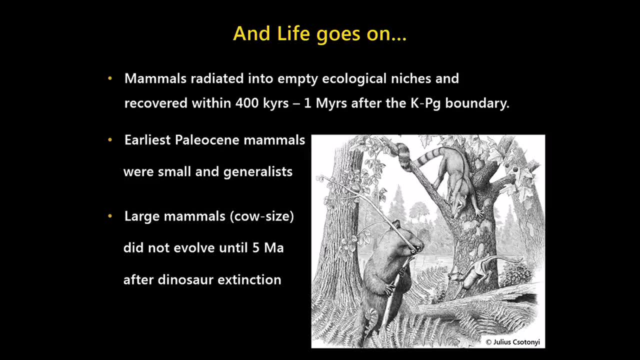 the mammal fauna has returned to pre-boundary diversity somewhere between 400,000 and 1 million years after the impact. So it definitely took longer for mammals to recover than for plants to come back. Earliest Paleocene mammals were very small and generalist, but then they. 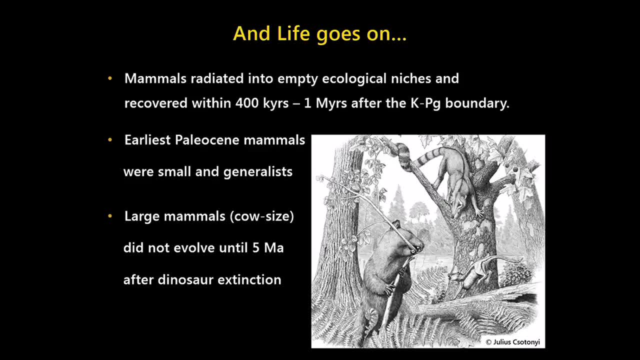 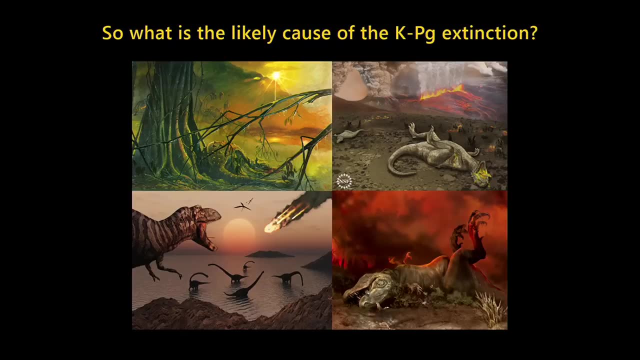 started growing back, but they didn't actually reach large size, like the size of a cow, until 5 million years after the impact. So it took a while for mammals to return to their former glory. So, in conclusion, what is the cause of the extinction of? 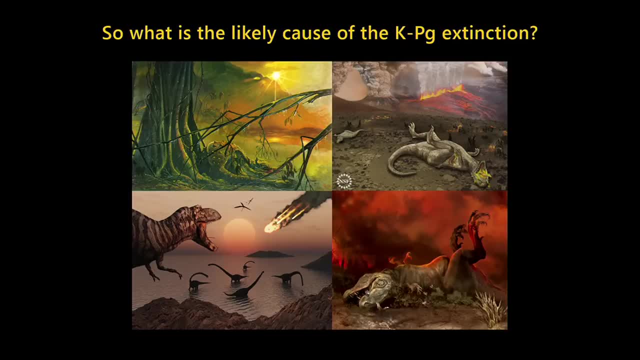 dinosaurs. We've seen a lot of various theories: climate change, volcanic eruptions, meteorite impact. Which one is responsible? Well, now it seems to be the consensus that actually it's not a single factor that caused the mass extinction. it's 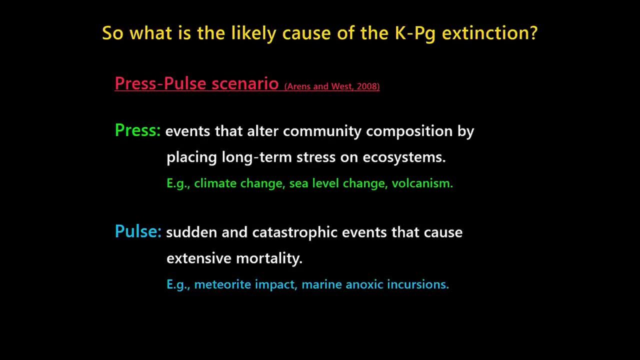 actually a combination of factors. That's the theory that we call the Press Pulse Scenario. It's been suggested in 2008 by authors that have split environmental factors into two categories. There's the press factors, which are long-term events that actually alter the community by putting 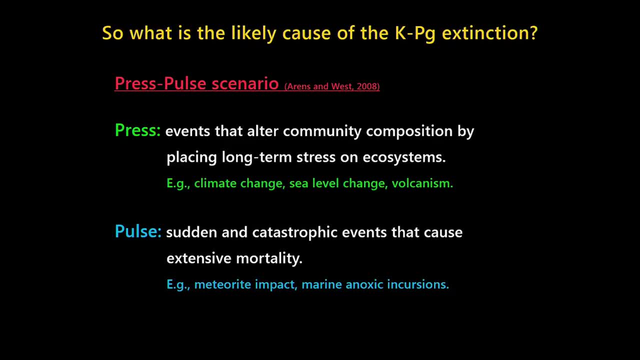 long-term stresses on the environment. So that can include climate change, volcanic eruptions and then the sea level change. So those long-term have a protracted effect on the environment. They put long-term stress on the environment And then you have 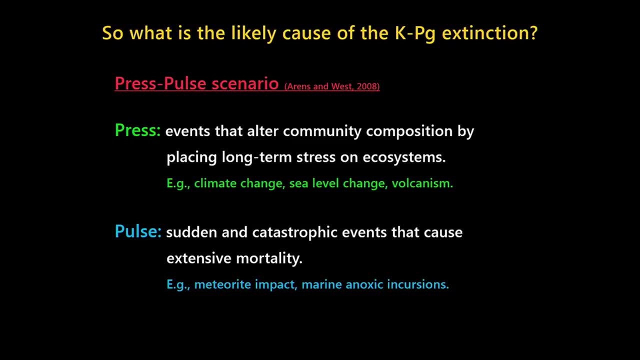 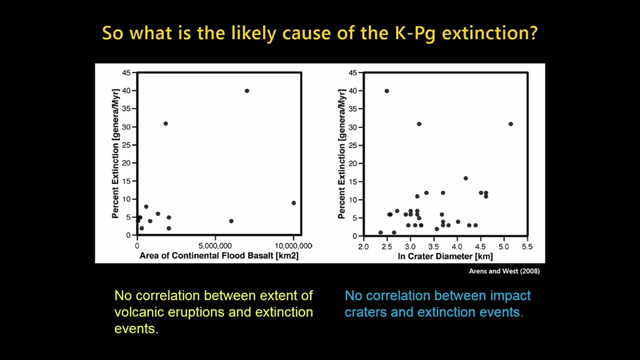 pulse events, which are sudden and catastrophic events that actually create a lot of mortality, And that includes events such as meteorite impacts, for example. So the authors decided to look at if there was a correlation between extinction events and volcanic eruptions or impacts. 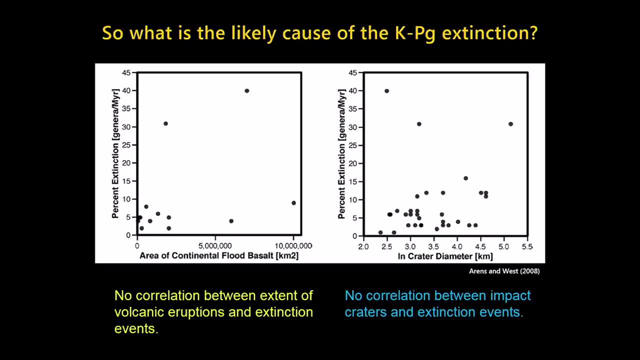 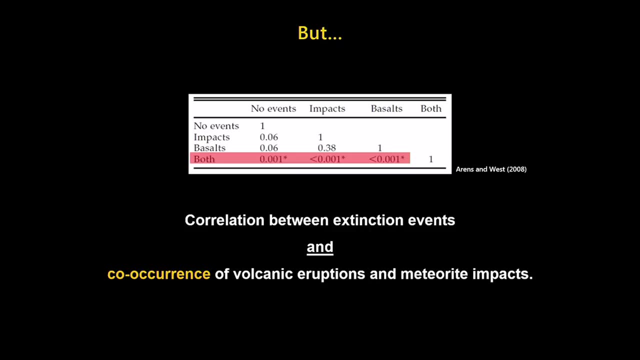 And they found no correlation between extinction events and eruptions, or extinction events and crater. But what they found instead is that actually there is a correlation between mass extinction events and the co-occurrence of volcanism and crater. So this means, when you have 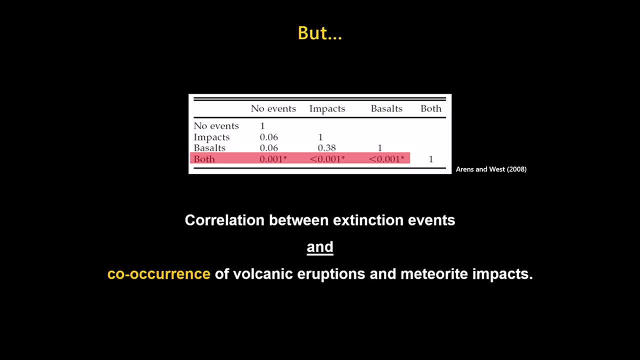 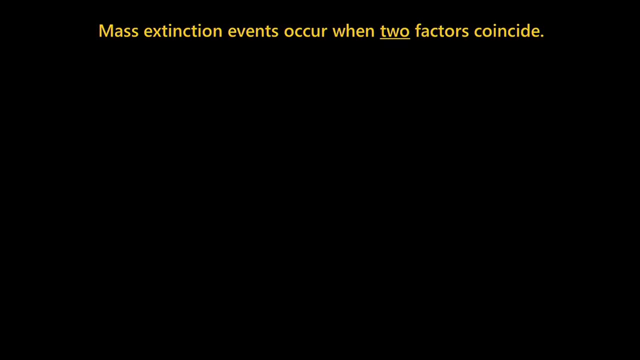 a long-term effect, for example, volcanic eruptions and a meteorite impact occurring in the same time interval that correlated positively with mass extinction. So their scenario suggests that basically, mass extinctions actually occur when two, press factor and pulse factor coincide. So in the case 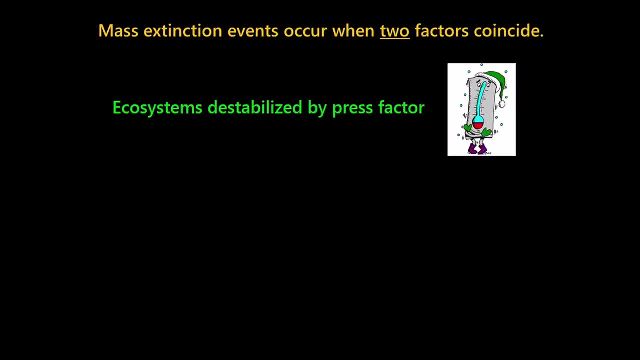 of the K-Pg boundary we have. ecosystems are being destabilized by the very rapid drop in temperatures- at least six degrees Celsius in mean annual temperatures. So that's destabilizing the ecosystems. They're trying to adapt to the changing climate And then you throw them a curveball.